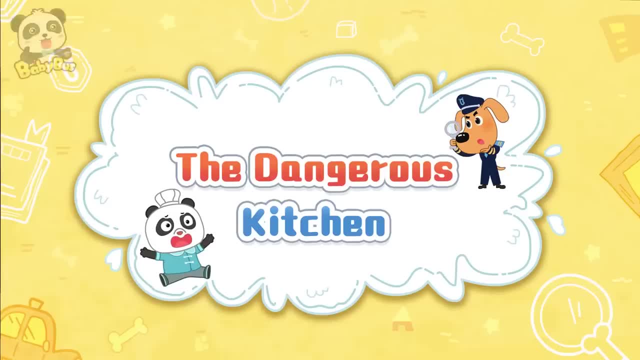 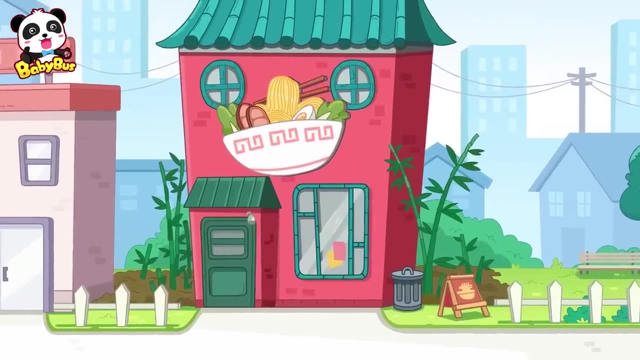 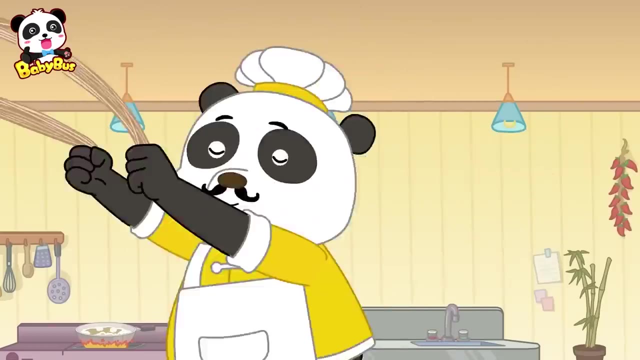 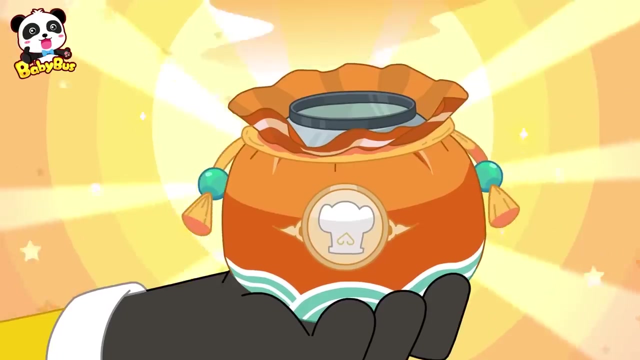 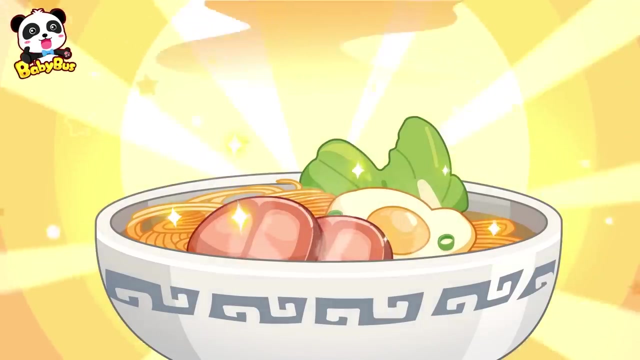 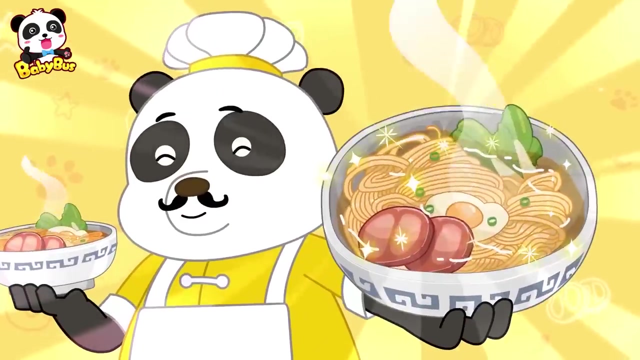 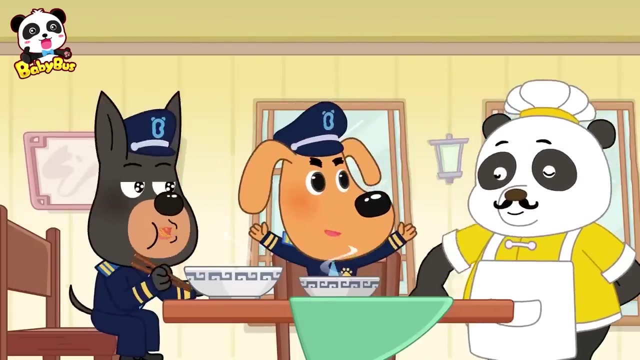 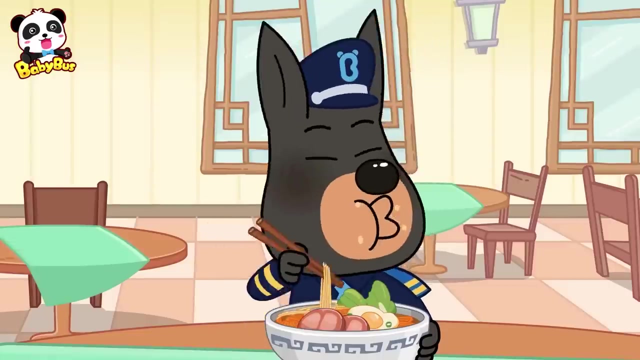 Baby Bus. The Dangerous Kitchen Smells so good. Two bowls of our signature noodles- Wow, It looks so yummy. Mr Panda, your noodles are amazing. That's because of our secret spice mix. Secret spice mix- Yeah, the recipe's from our daddy's, daddy's daddy. 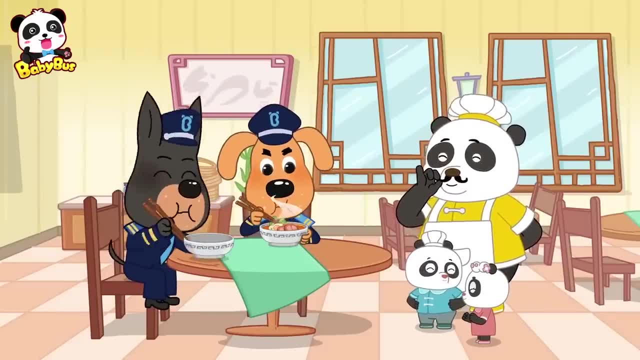 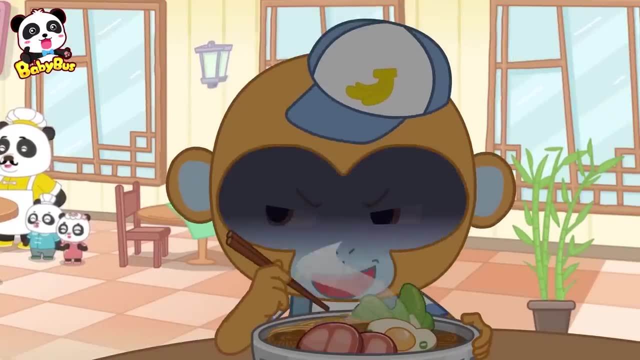 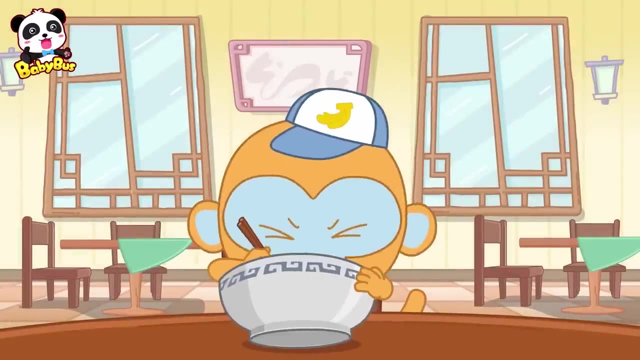 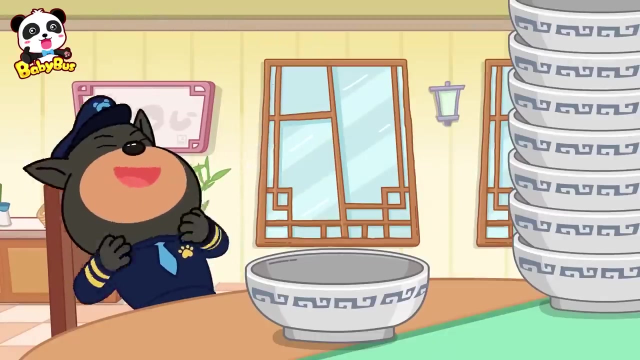 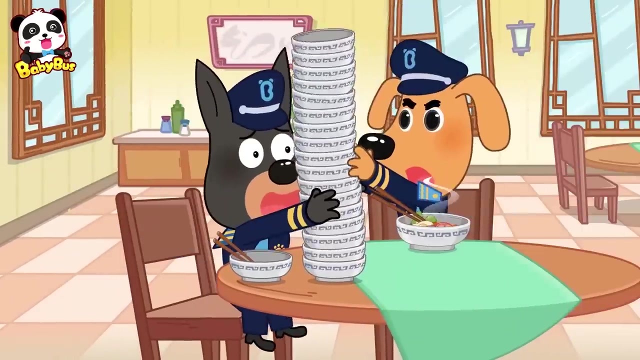 That's right. Another bowl please. If I had the secret spice mix, I'd be able to make yummy noodles too. Amazing. Another bowl please, Mr Panda, My spice mix. What happened? Let's go and have a look. 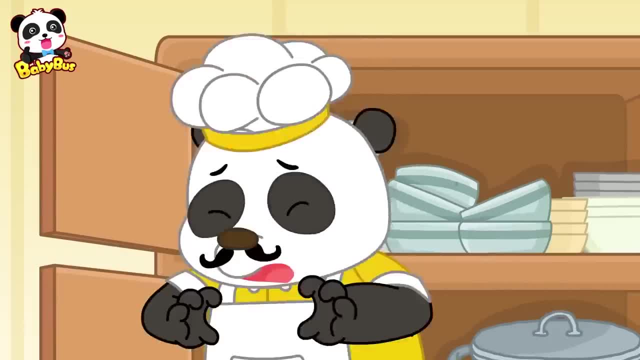 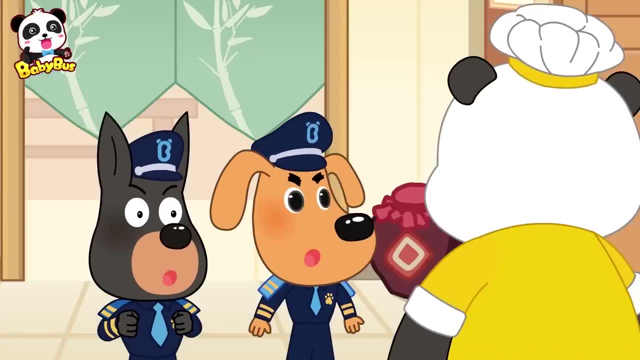 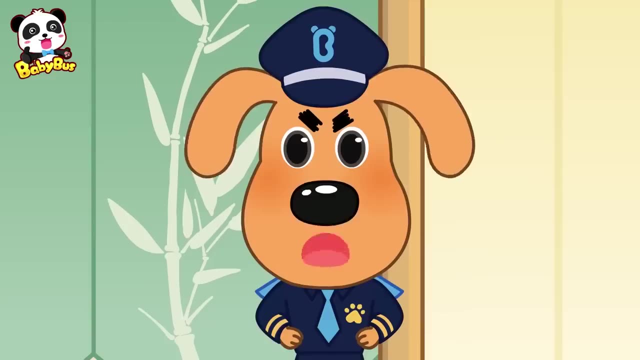 Mr Panda, what's wrong? Sheriff Labrador, my secret spice mix is gone. What It's handed down to me by my family and now it's gone. Please help me find it. Oh, Don't worry, There's no case that I can't solve. 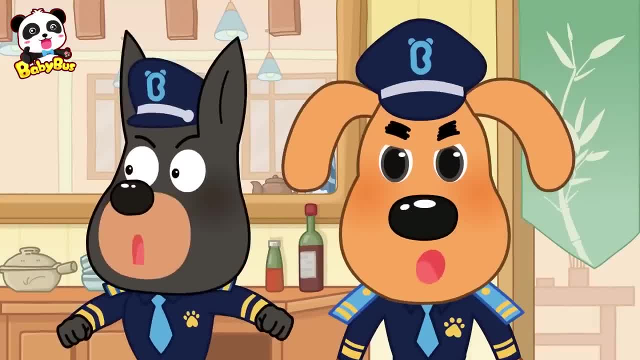 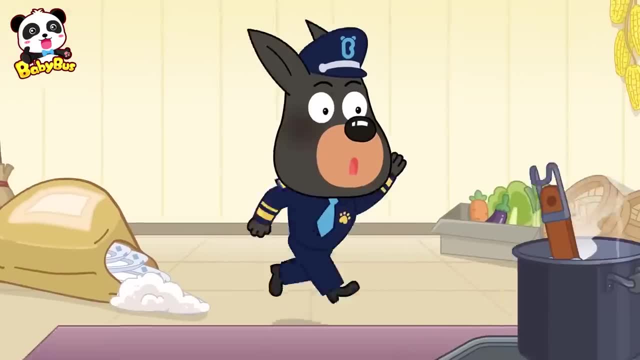 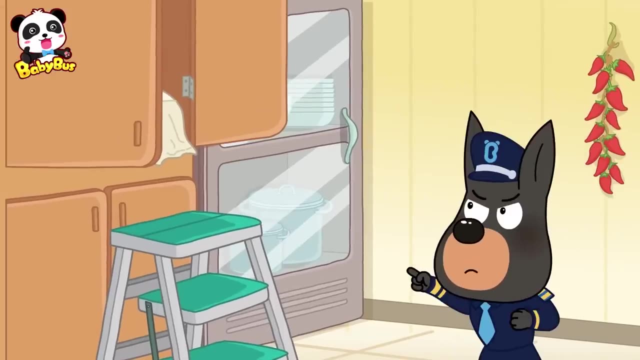 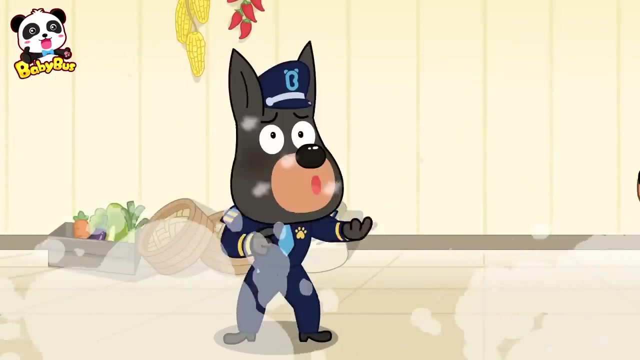 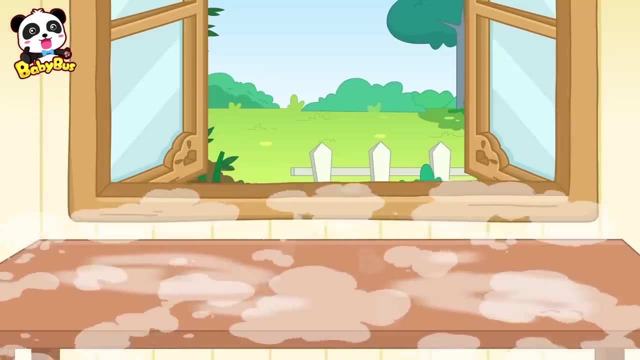 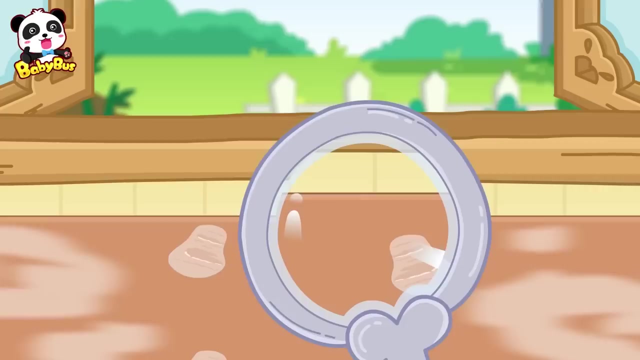 If it was stolen, there must be clues left around here. Dobby, let's split up and look around. There's the thief. Huh, It's just flour. It's just flour Footprints. It looks like the thief broke in through the window. 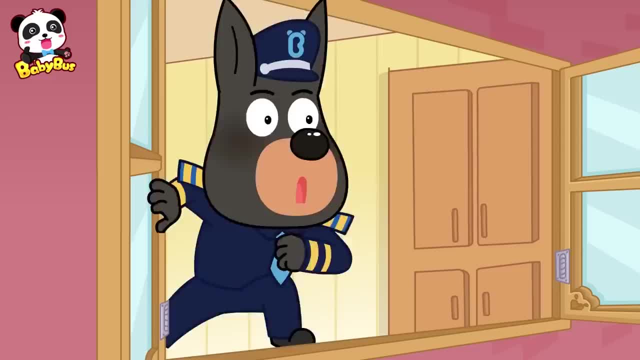 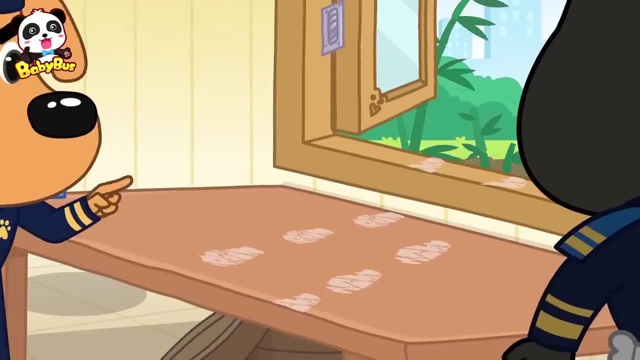 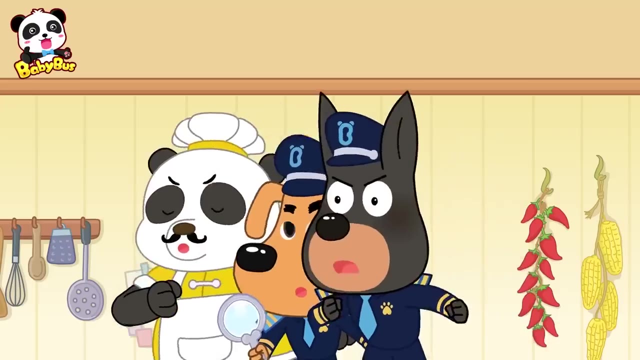 Unbelievable. I'm gonna catch the thief. Wait, The thief might still be here. What, What, What? Look, there were no footprints leading out of here, So the thief must still be here. You can't run away. 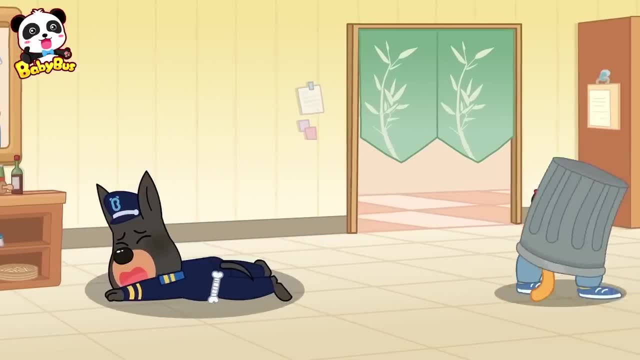 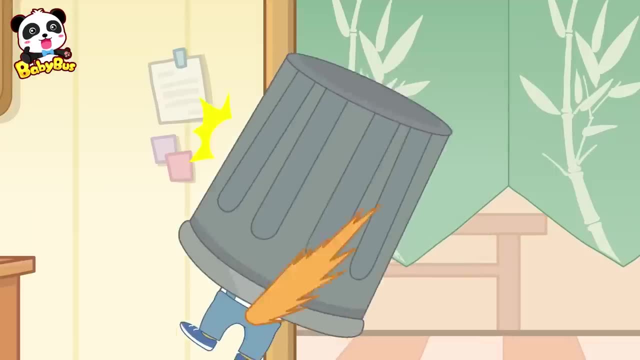 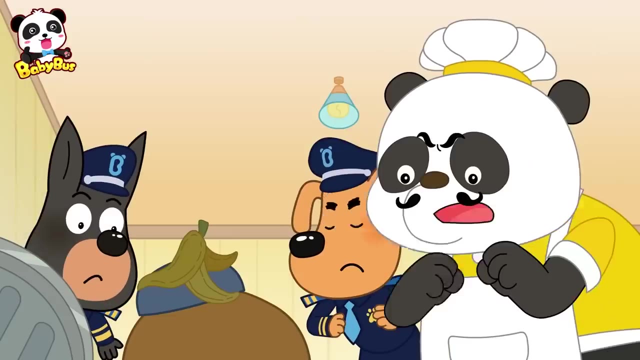 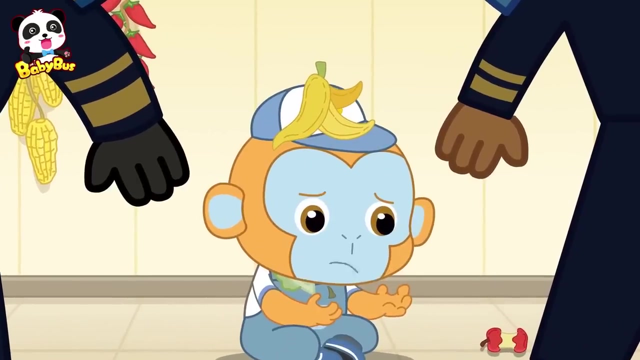 I got you. Ouch, Stop right there. Stop right there, Mr Monkey. Mr Monkey, It was you, It was you. Ah, Oh, No, It wasn't me. I'm sorry. I just wanted to see how the noodles are made. 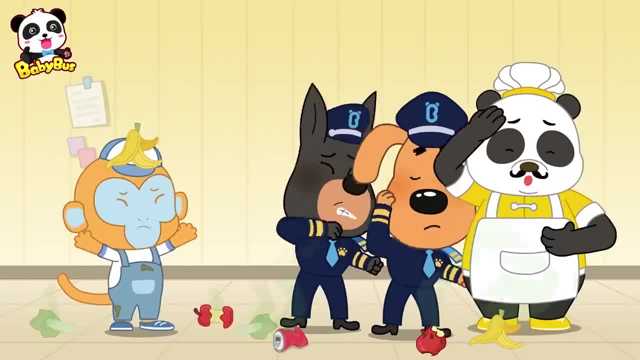 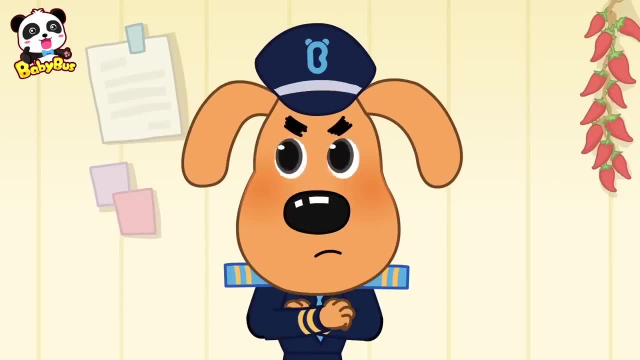 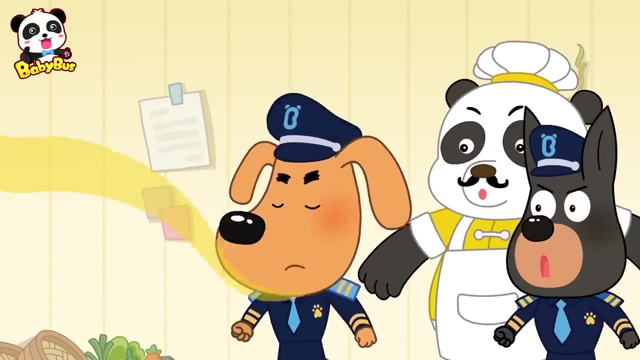 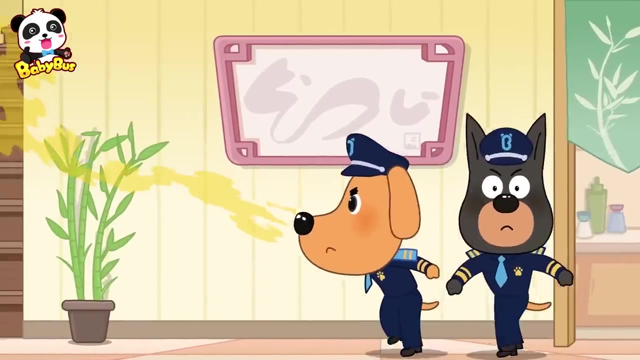 I didn't steal your spice mix. You can search me if you want. If it wasn't Mr Monkey, then who was it? Huh, I think I smell the spice mix. Follow me, Huh, The smell's coming from up there. 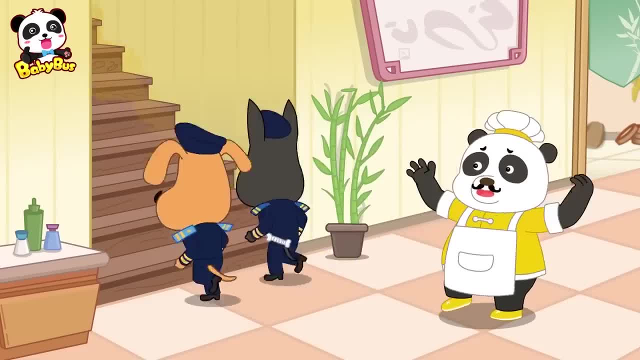 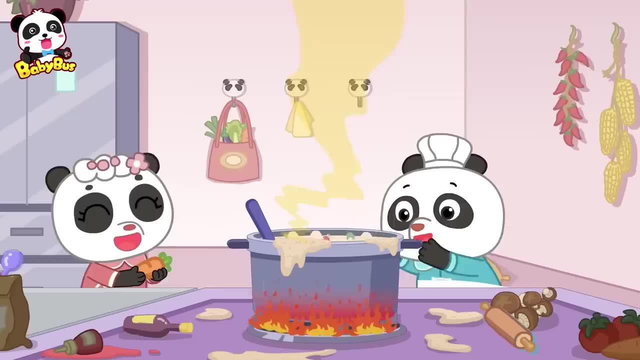 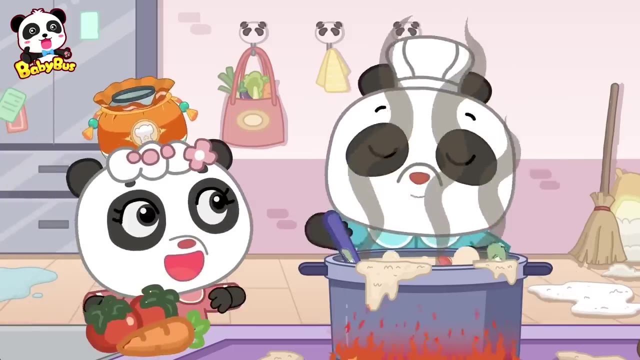 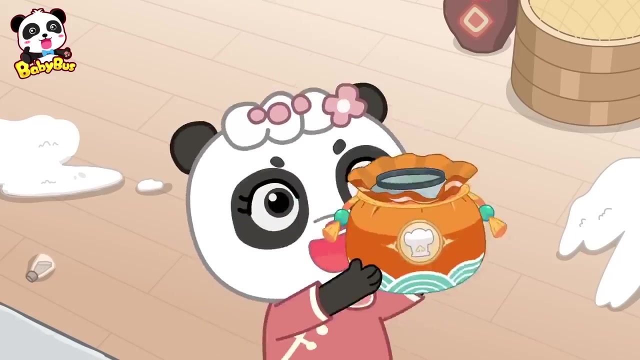 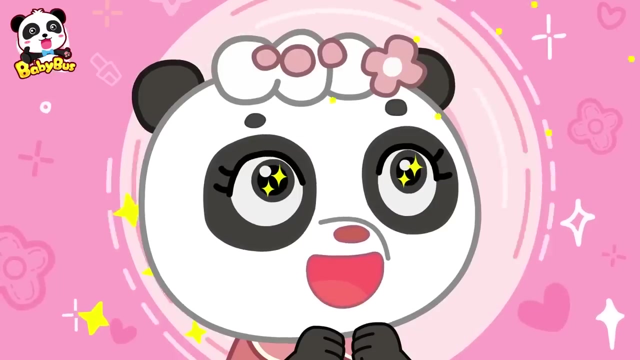 There's another kitchen upstairs. Come on, let's go. Tomato, Carrot, Mushroom, Cucumber- I'm the best chef in the world. Wow, Mr Chef, The secret spice Here. Wow, Ow My eyes. 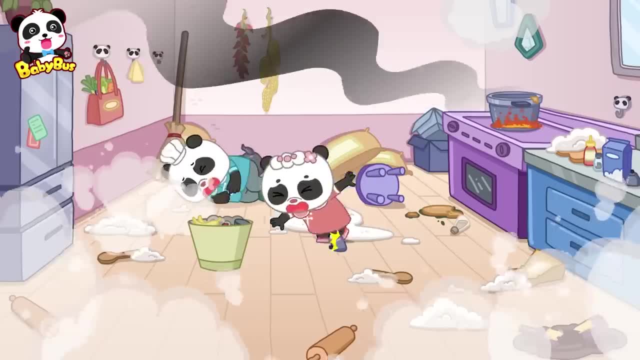 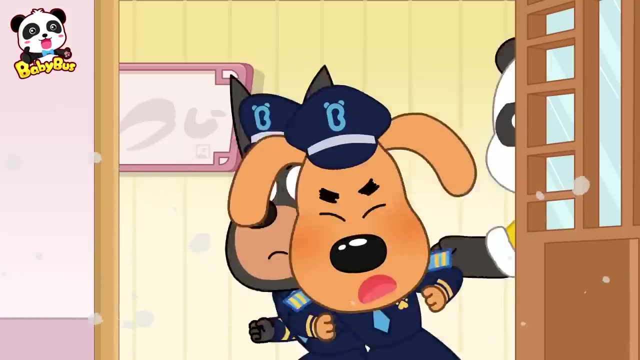 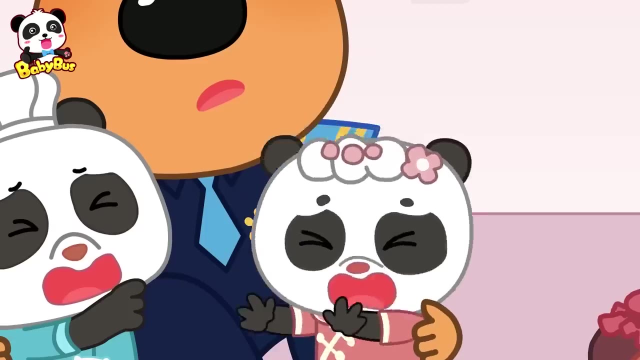 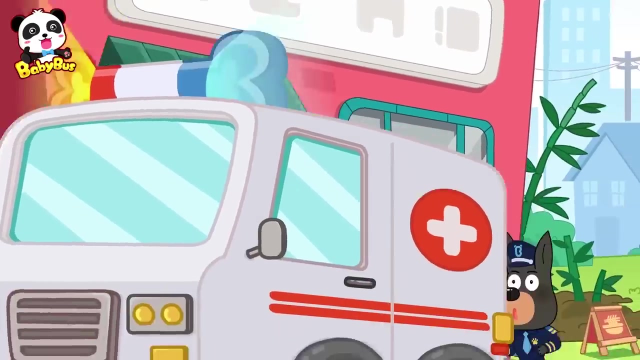 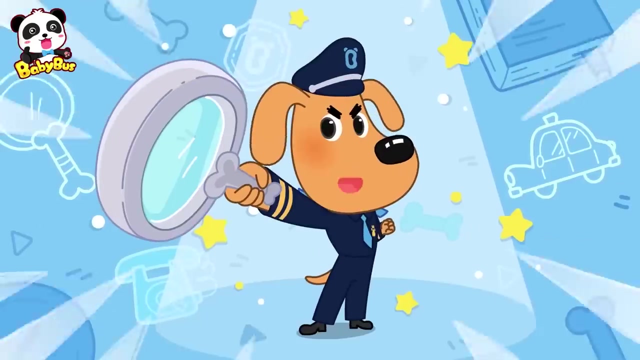 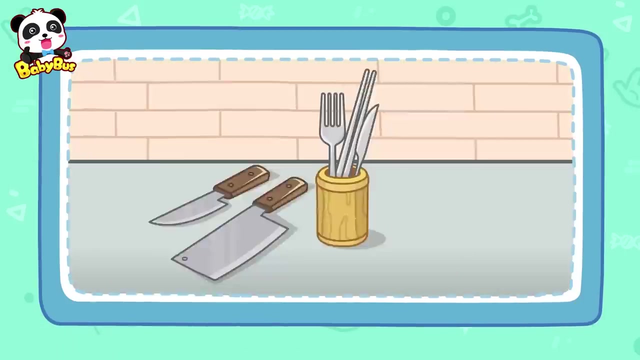 It's my daughter. Hurry, Watch out. Let's go My eyes. We need to send her to the hospital right now. Phew, Sheriff Labrador's Safety Talk. Kids never play in the kitchen. There are sharp knives and tools. 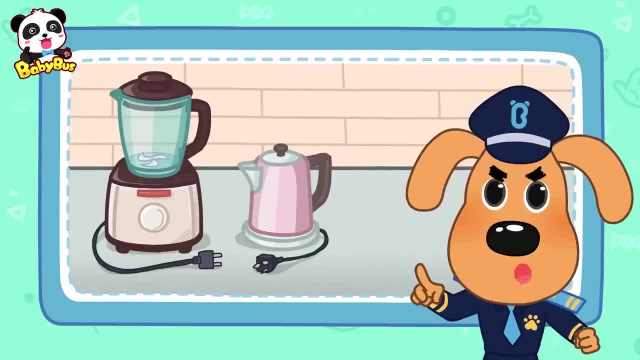 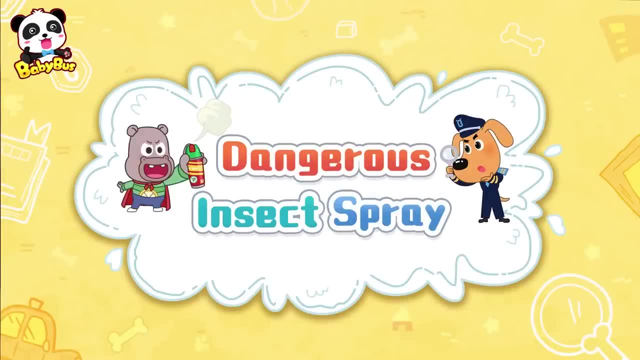 boiling water and electric appliances in the kitchen, and they can hurt you Also. parents need to keep an eye on their children when they're in the kitchen too. Woof, Dangerous insect spray. Wow, It's so yummy, Oh no. 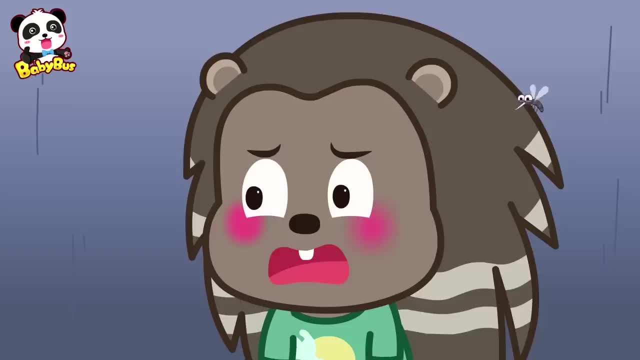 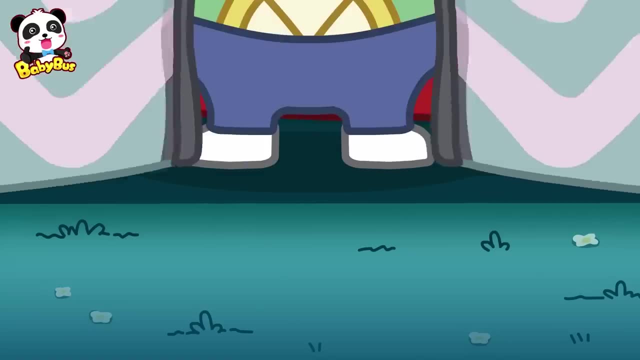 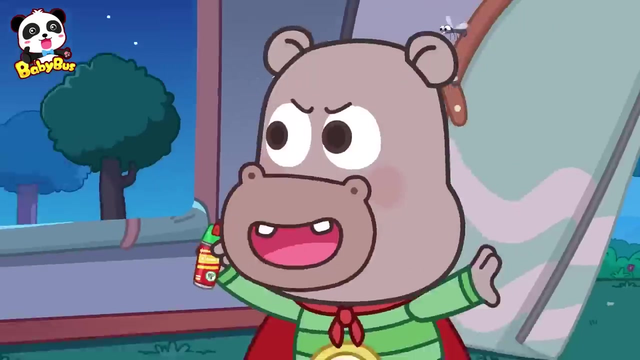 The skittles, Oh Ouch. Ah, You won't wear a skittle, Don't go away. Hey, Ha-ha, Super skittles, A skittle hunter can get rid of every mosquito, Oh Ha. 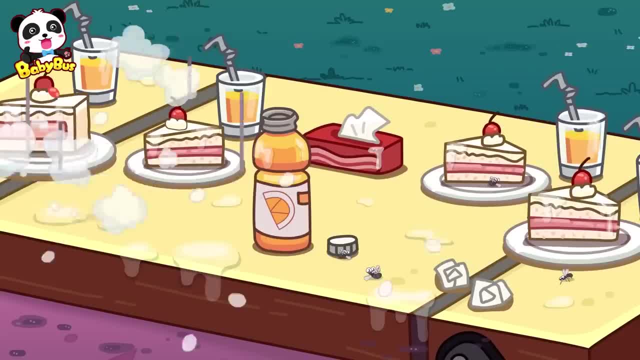 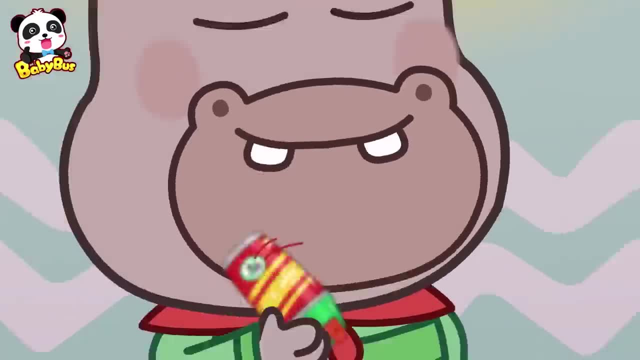 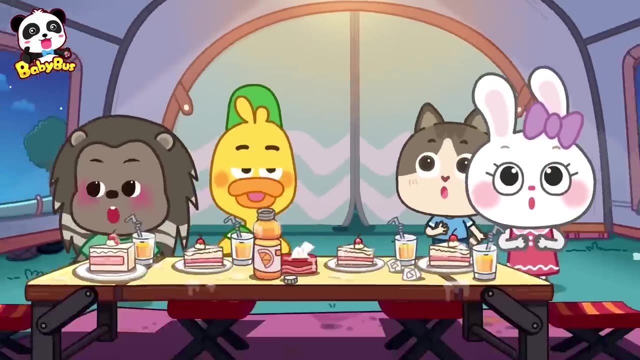 Good, Whoa, Ha-ha, Whoa, What, Whoa, Ah, Whoa, Mission complete And you're welcome. Whoa, Oh, Oh, Yay, Two more mosquitoes, Yay, Ha-ha. 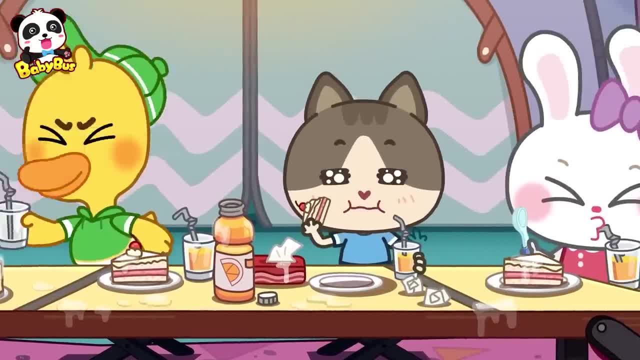 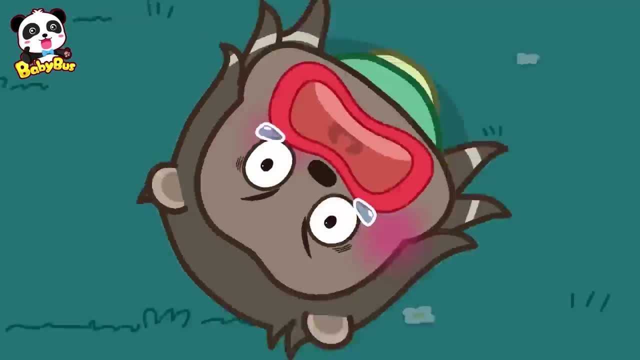 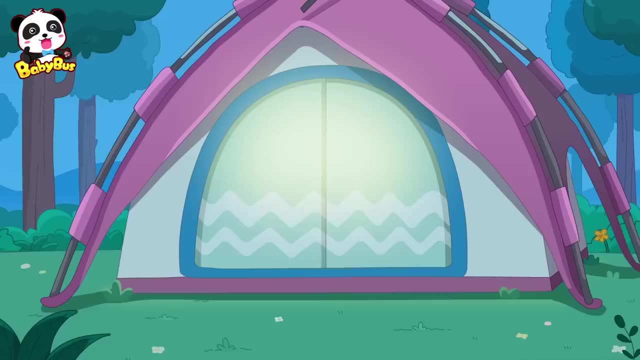 Let's see: Ah, Ah, Ah, Ah, Ah, Ah, Oh, my tummy hurts, Ah, My tummy, Oh, Ah, Ah, My tummy, Ah, Ah, Uh, Oh, Ahh, Oh. 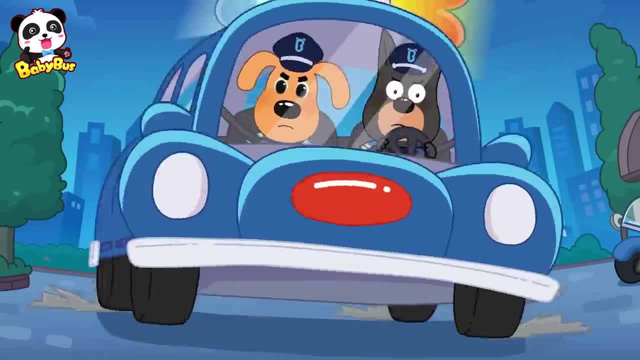 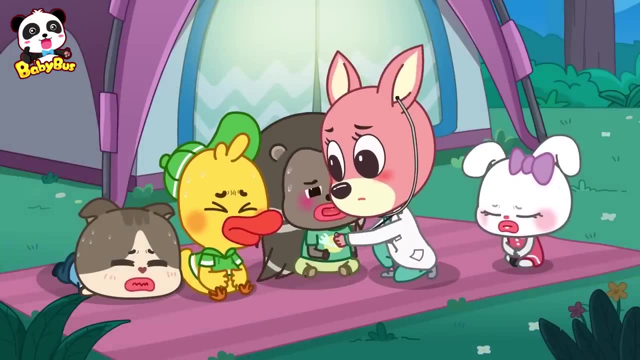 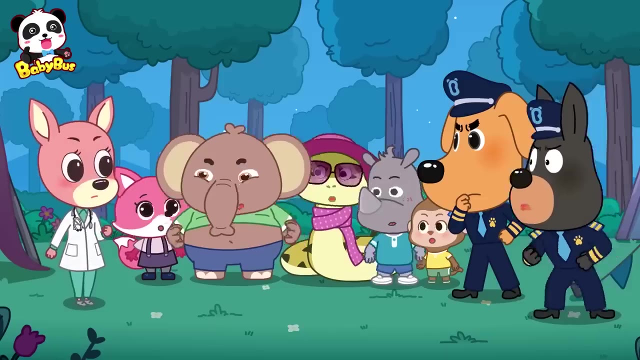 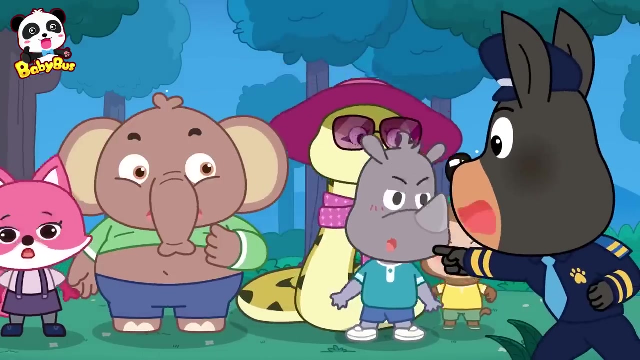 Ah, Ow, Ow, Ow, Ah, Oh, Oh, Oh, Ah, Ow, Ow, Oh Ow. Sheriff Labrador, the children seem to be poisoned. What They're poisoned, It's a viper. What? No, not me. 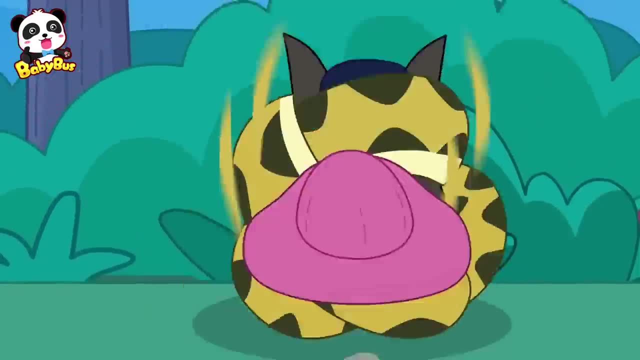 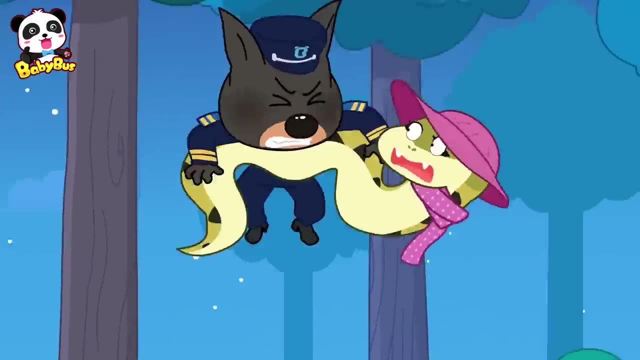 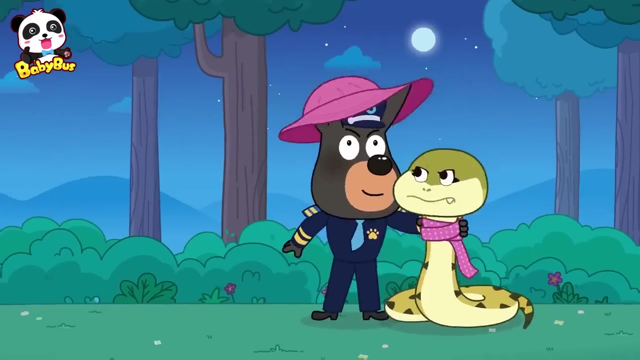 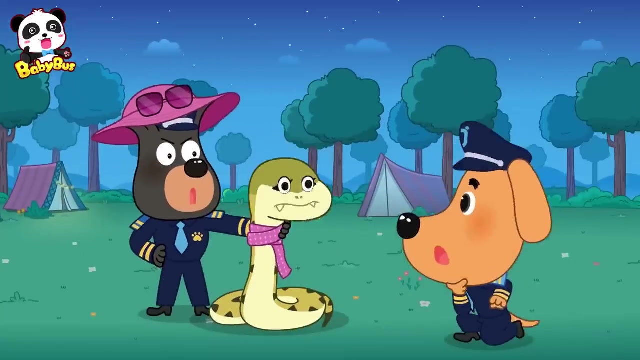 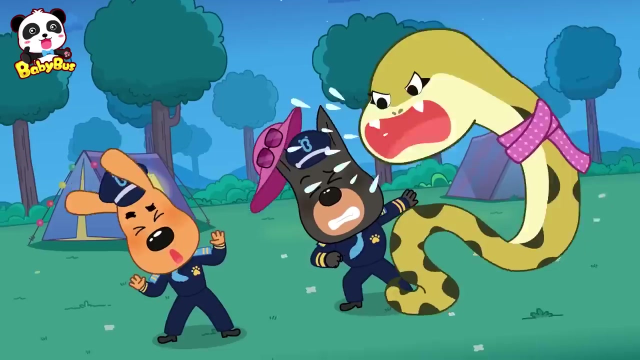 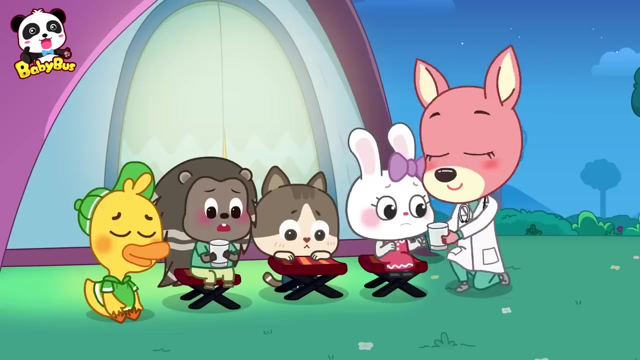 Stop right there. Look at these big fangs. She must have bitten the children. Well, Dobie, this is a king rat snake. We king rat snakes are not venomous. I'm so sorry There's no wound on their bodies. 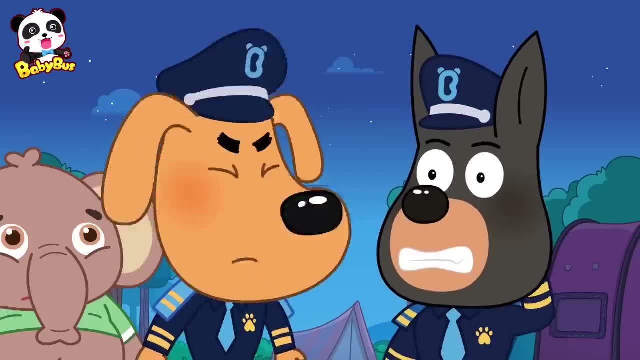 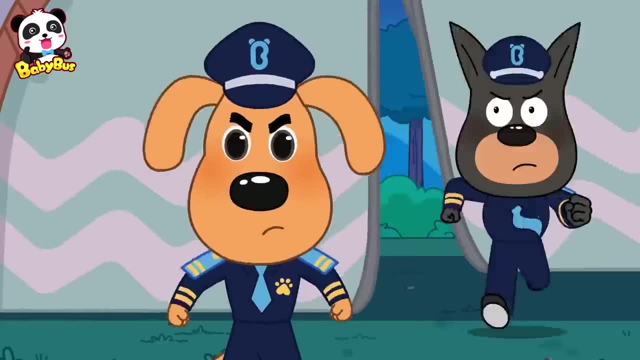 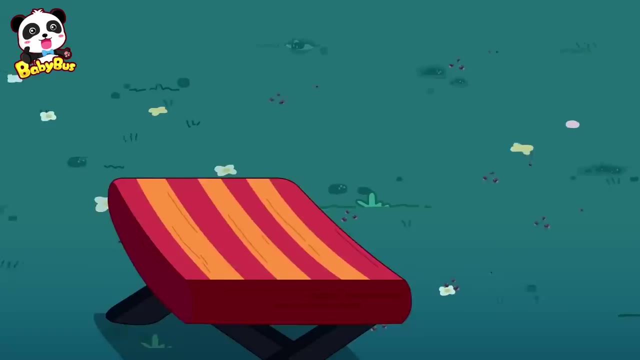 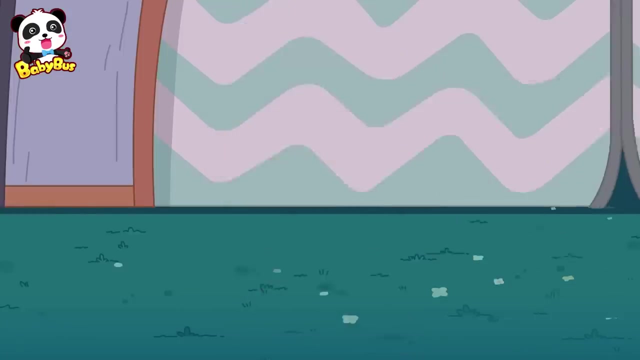 I don't think it's a venomous animal that attacked them. If it's not an animal, what made them sick? then Let's investigate the scene. What's that smell So many mosquitoes? Hey kids, did you use insect spray just now? 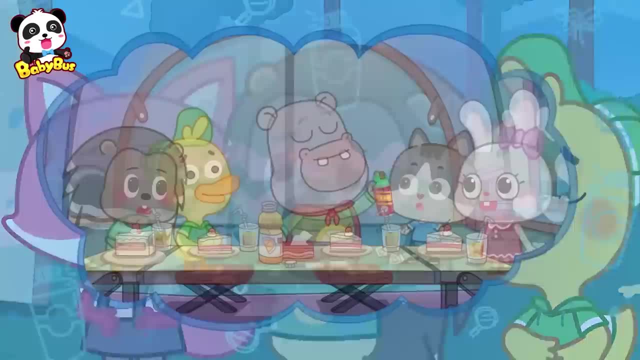 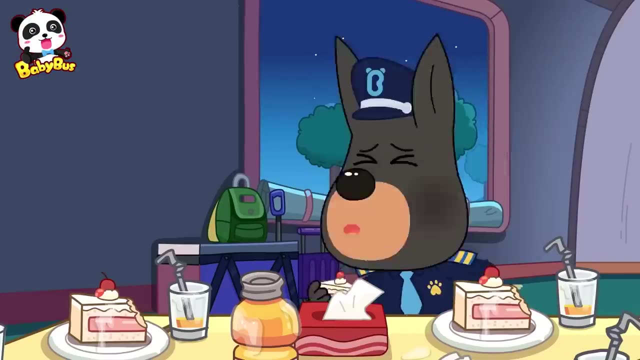 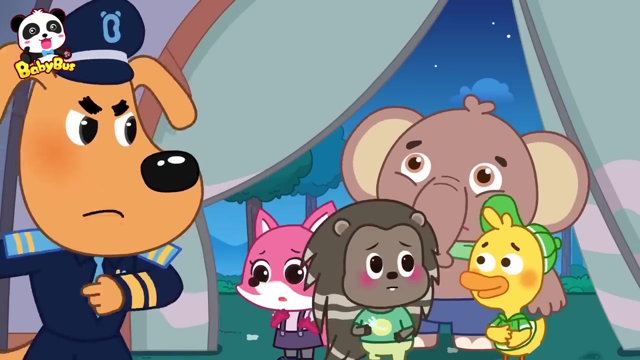 Uh-huh, There were a lot of mosquitoes in here, so Little Hippo helped us out, Got you. The cake smells like insect spray too. Insect spray is toxic. You must have been poisoned by the cakes covered with insect spray. 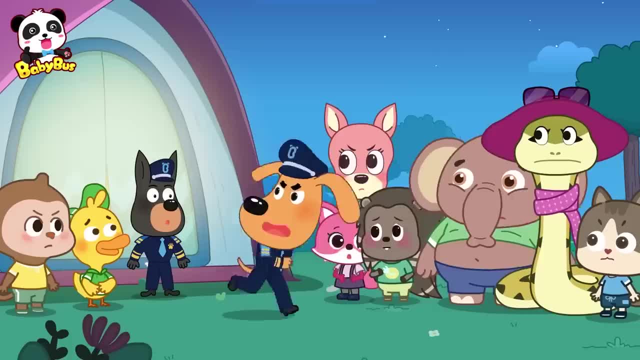 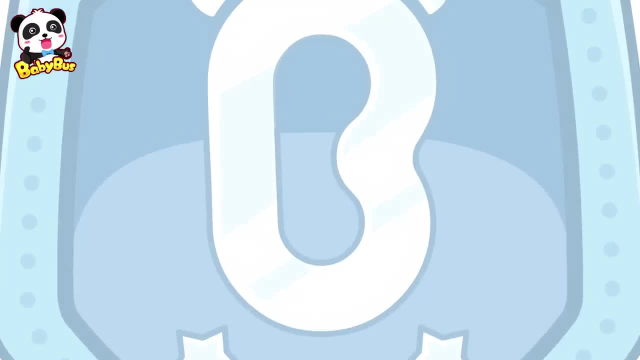 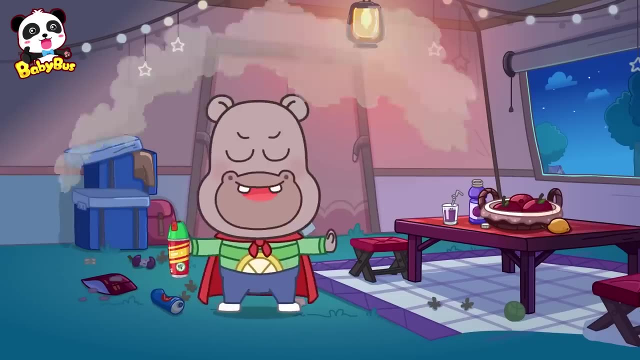 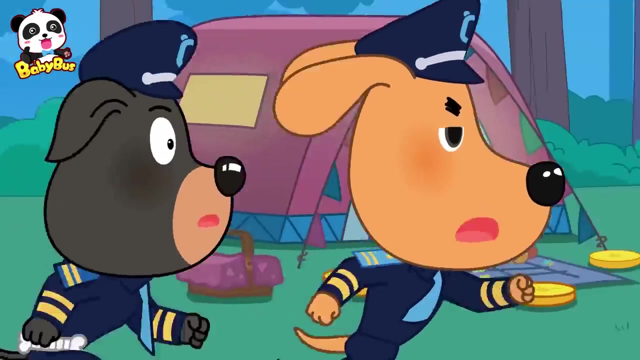 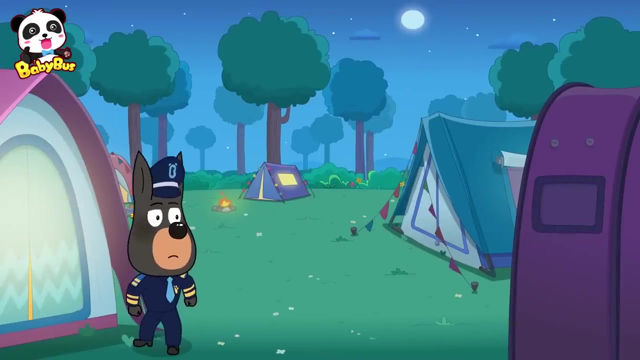 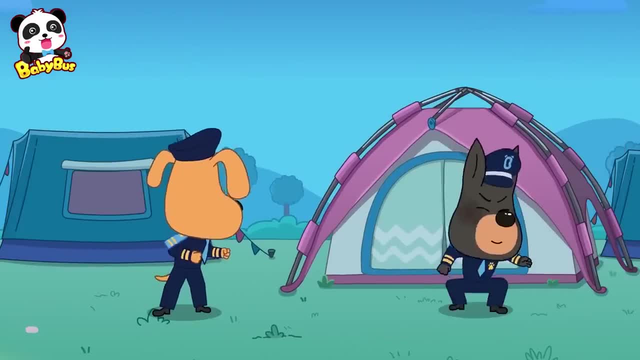 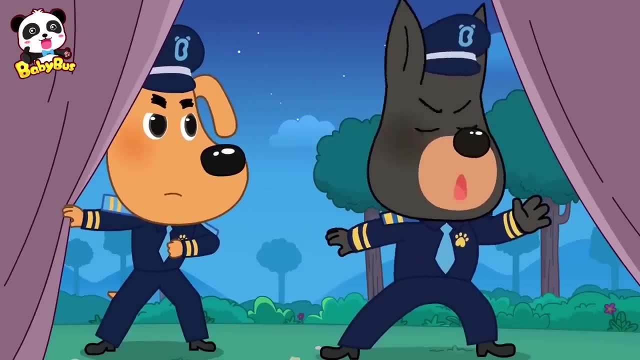 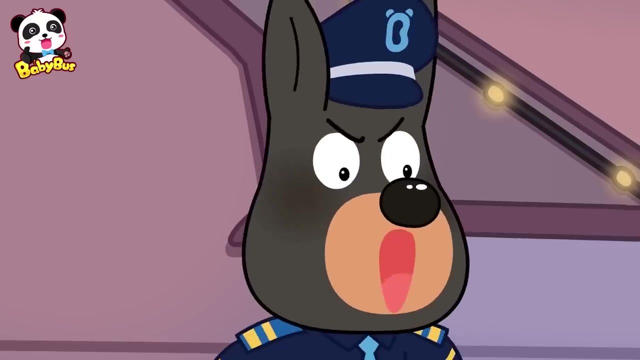 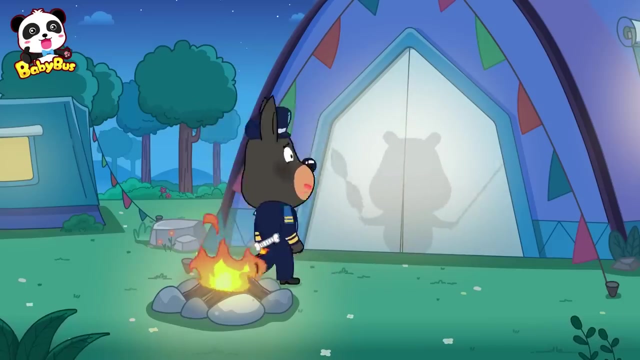 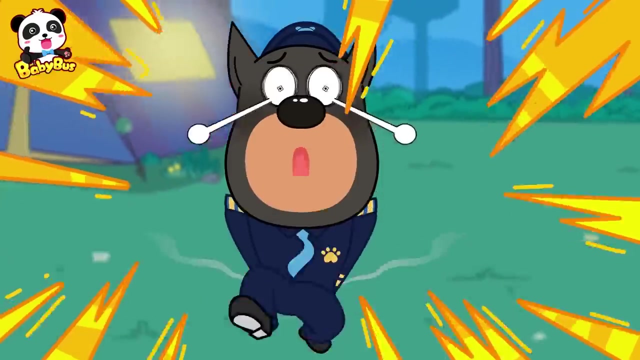 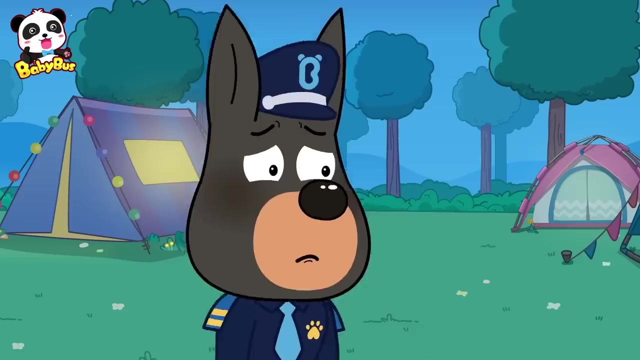 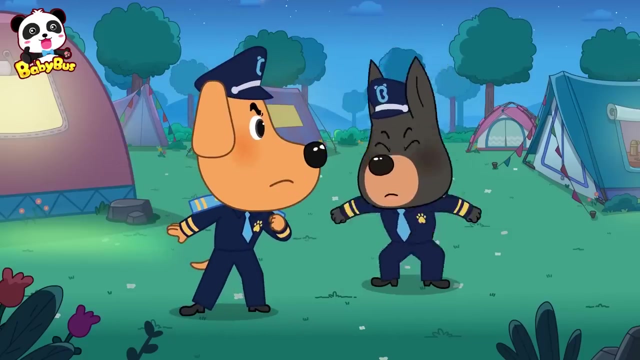 coming, coming, coming. I found him Here, Little hippo, I'm little hamster. I'm so sorry, Wrong person Here, So hot. What's that smell? It's my burned tail And insect spray too Over there. 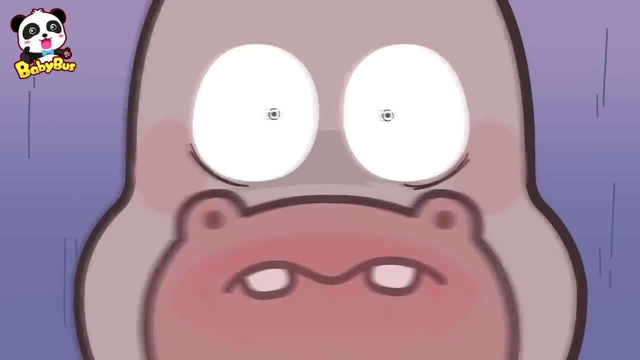 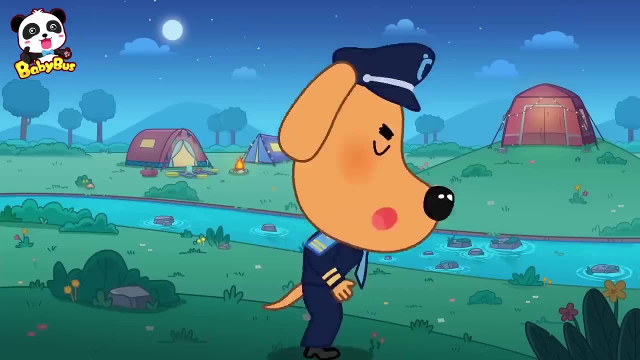 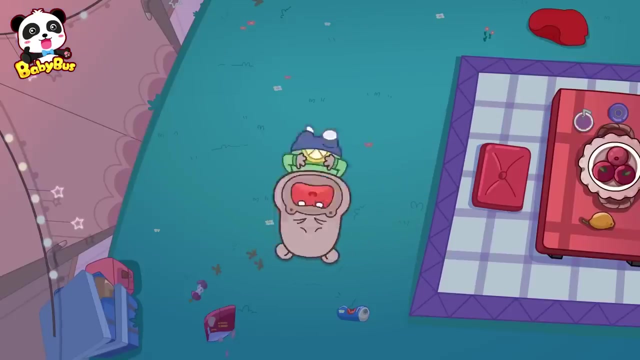 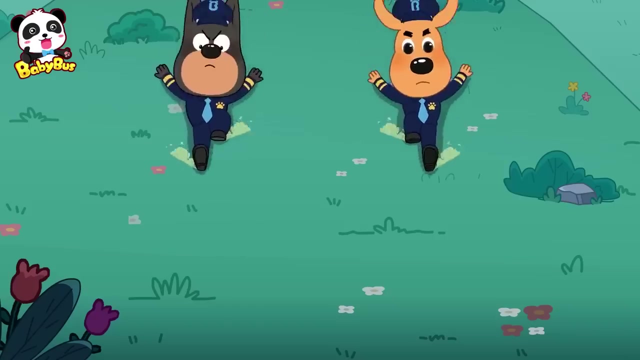 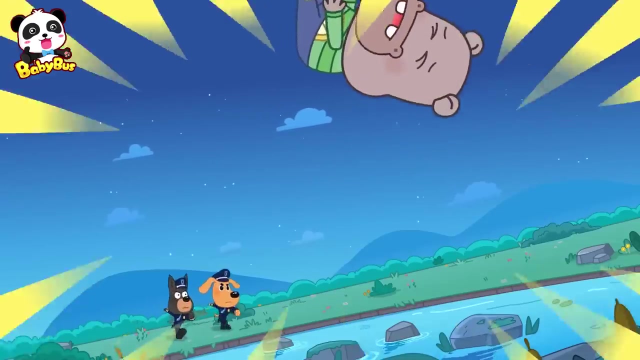 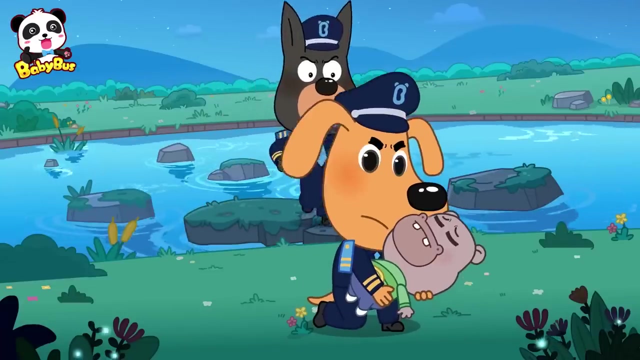 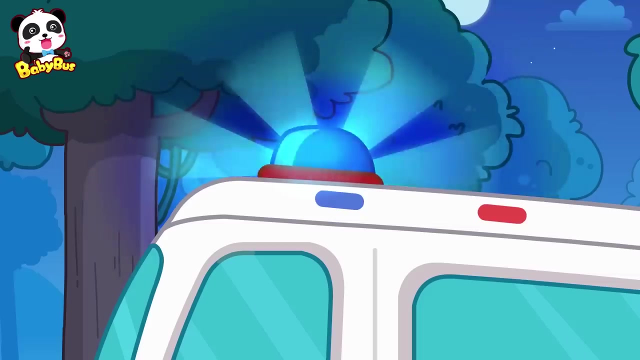 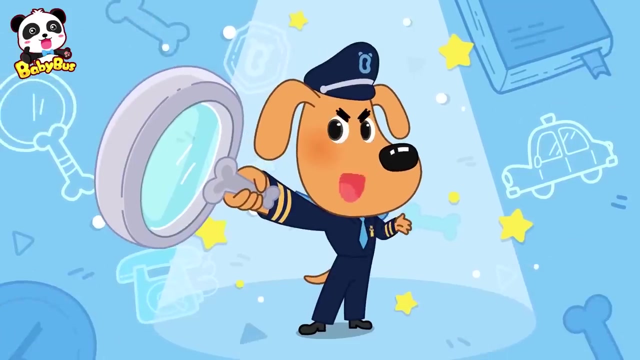 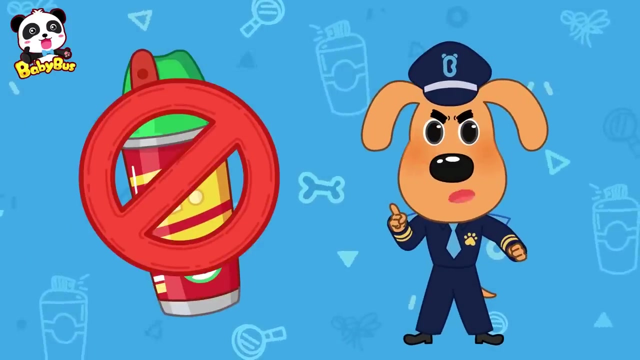 My tummy, My tummy, Over there, My tummy, Oh no, Whoa, Little hippo, Little hippo, Let's take him to the doctor now. Sheriff Labrador's Safety Talk. Kids. Insect sprays are toxic. 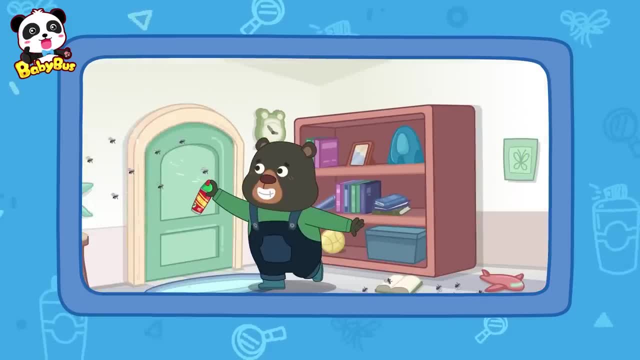 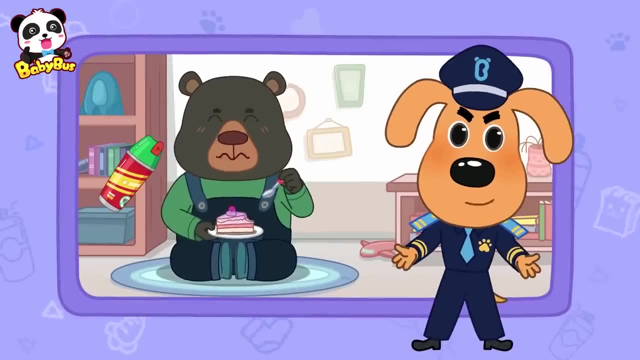 You should be careful when using them. If you have to use insect spray, quickly leave the area after spraying it, Change your clothes and wash your hands. Also, you shouldn't spray it at people or on food, because it might harm others and even yourself. 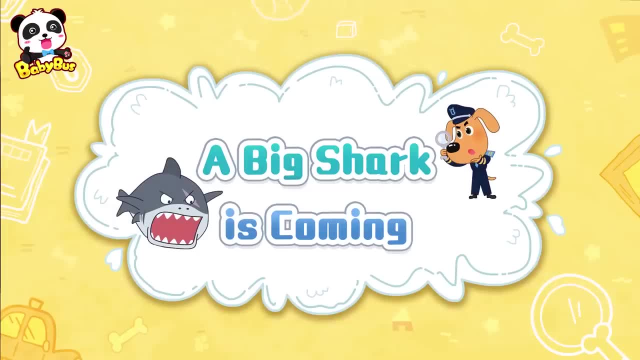 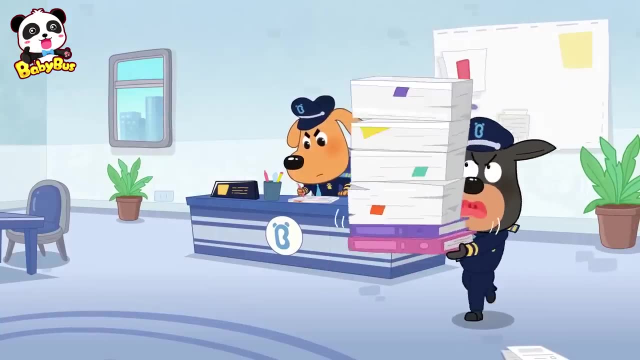 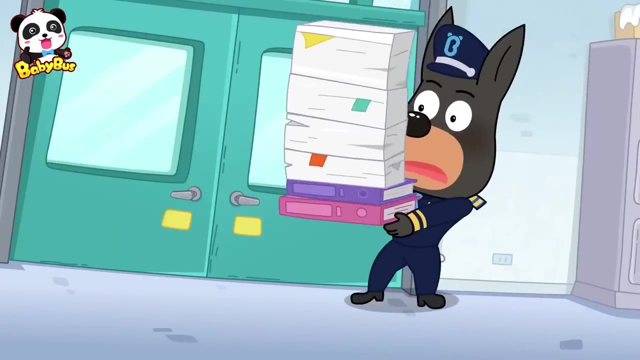 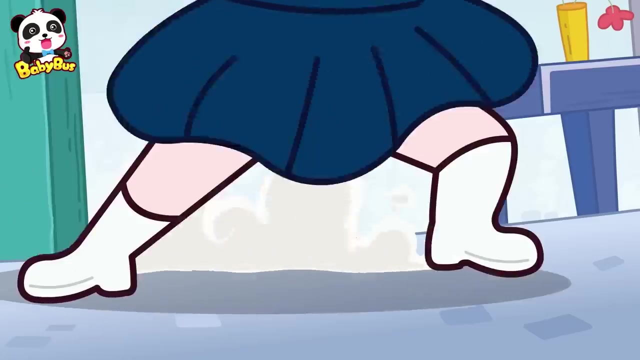 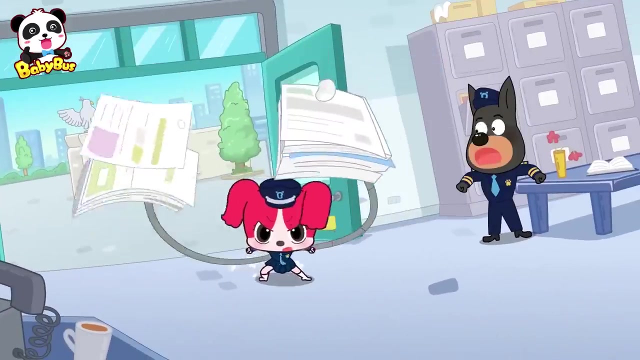 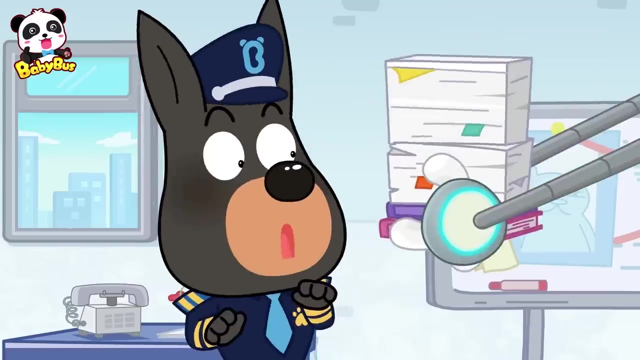 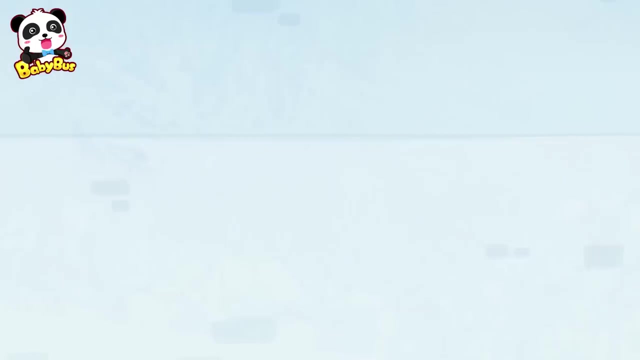 Please remember that A big shark is coming And little hippy is coming too, Don't worry. Wow, Here you are. Ha Ha Hi, I'm the new police officer Papillon. Nice to meet you, Officer Papillon. 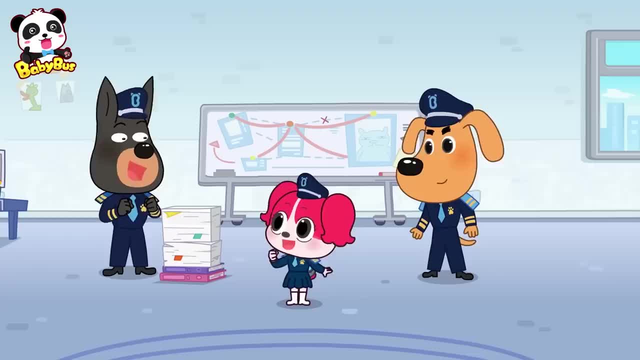 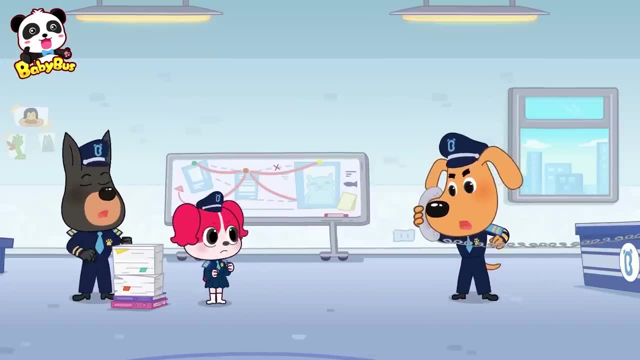 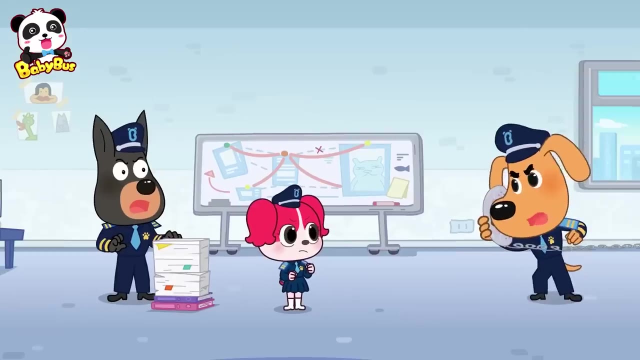 I have lots of useful tools. They'll be handy for operations. Woof, Hi, I'm Sheriff Labrador. Sheriff Labrador, a shark is biting people. Please come A shark, Hello, Hello. Let's go to the beach right now. 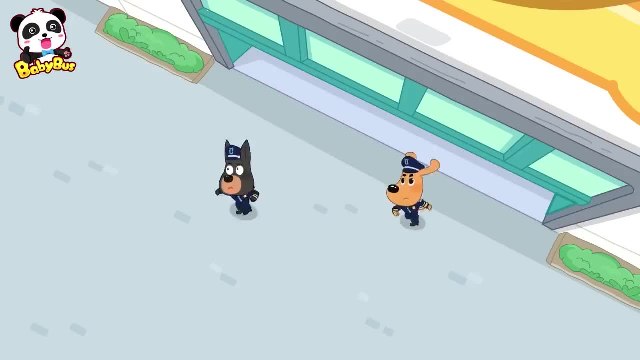 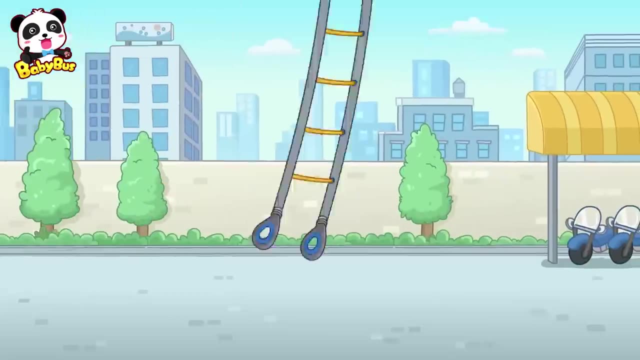 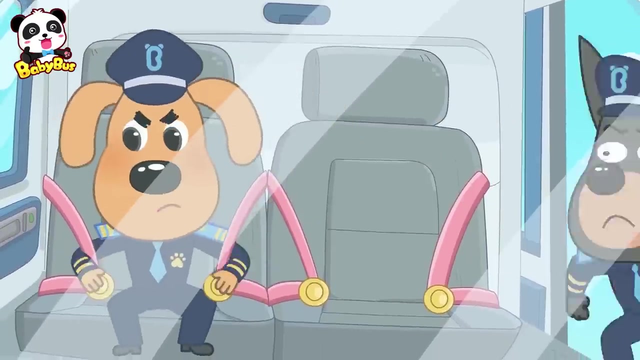 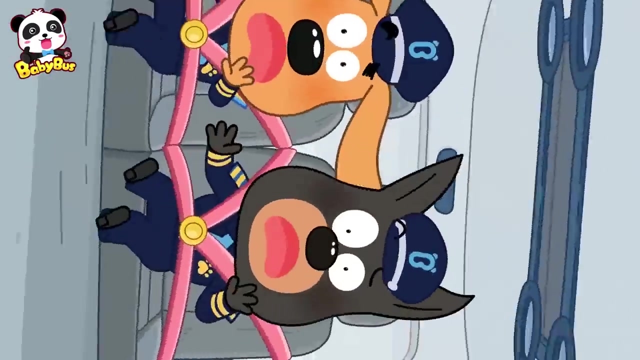 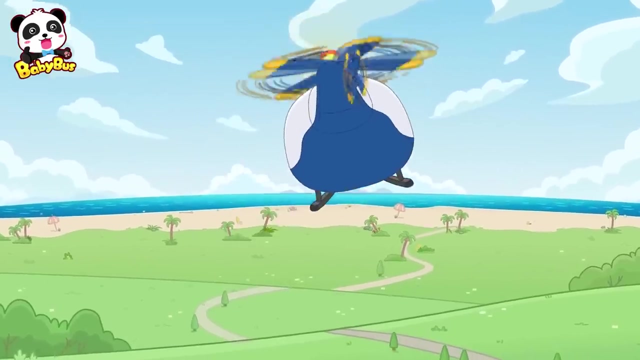 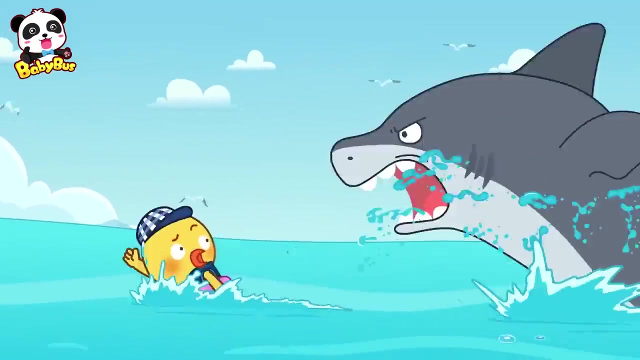 OK, Ah, so windy. Come on up, Hold on tight, Look what I've got. Spin spin Up into the sky. Ah The shark. Ah, Dobby, let's go Watch out. Ah, Watch me. 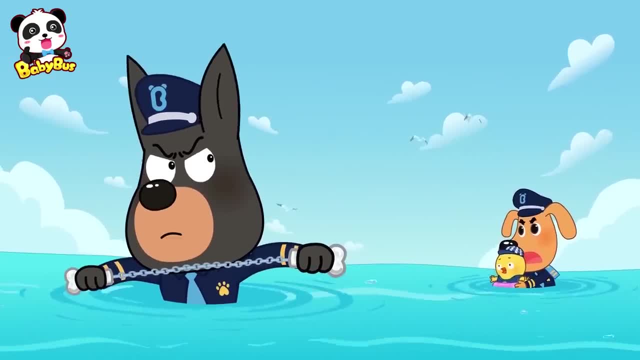 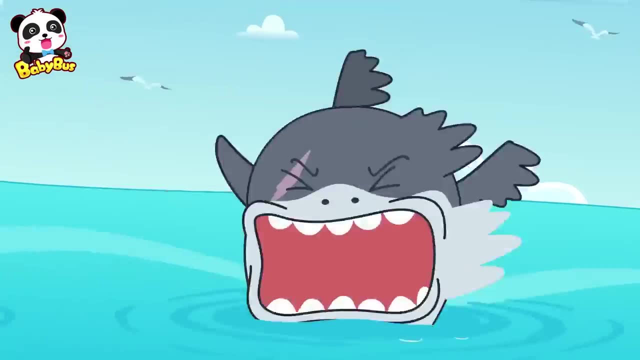 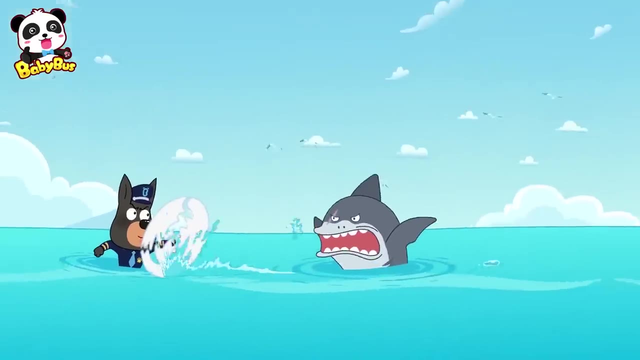 Wadda Go, I'll take care of the shark. Thanks, Dobby. Ah, Everyone, get out of the water right now. Ah Ah, Eat this. You can't bite me. Wadda Wadda. 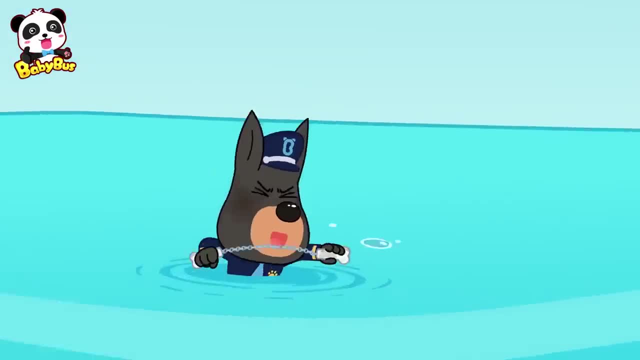 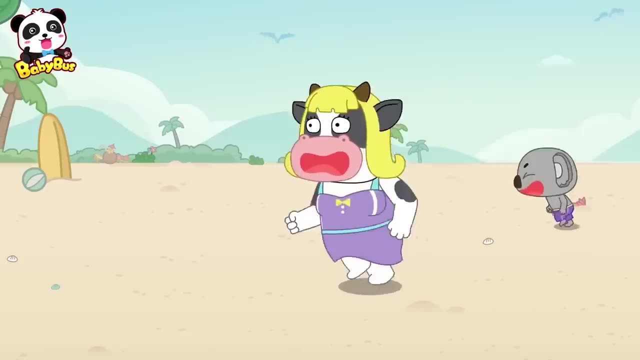 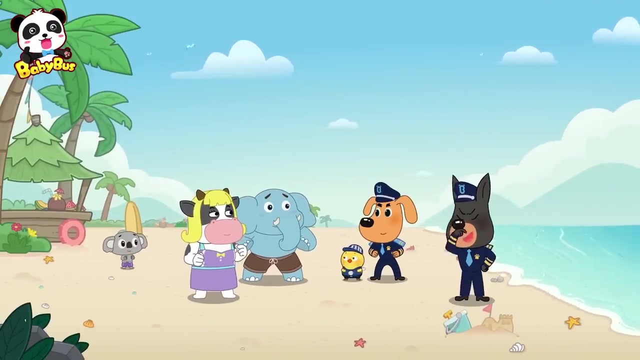 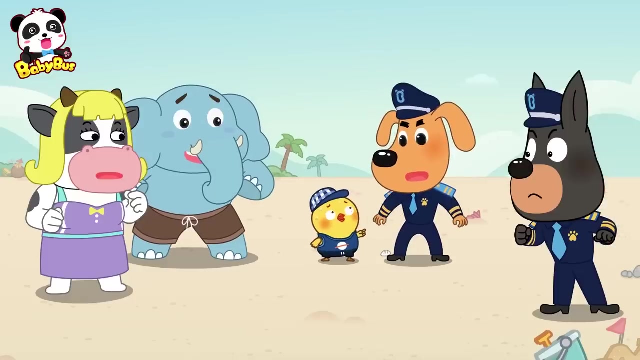 Dobby, come on up now, All right, Ha, Roughly time's over. Bye-bye. That was so scary. Thanks, You guys are awesome. Sheriff Labrador, my brother went out surfing, but he isn't back yet. 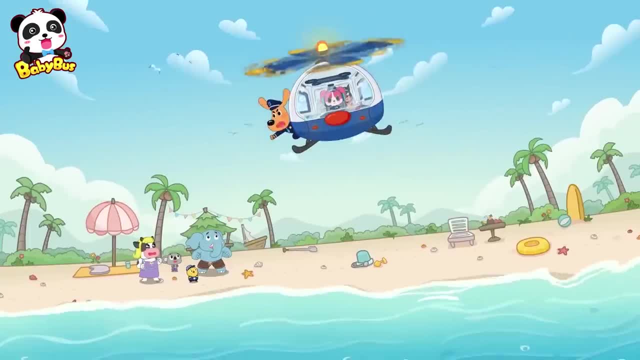 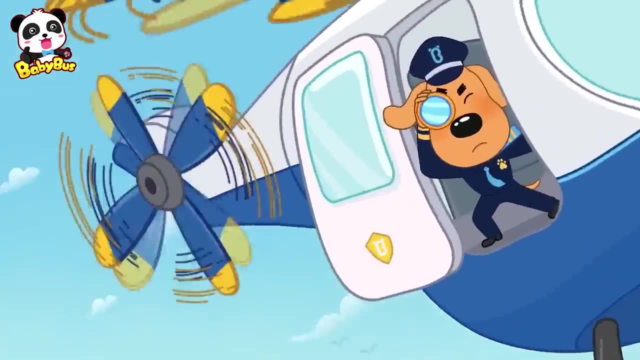 What? We'll go find him right now, All right. All right, We'll be right back. We come back when we're saved. All right, etus, how have you been? Where's your girlfriend? Who Don't feel internationally? 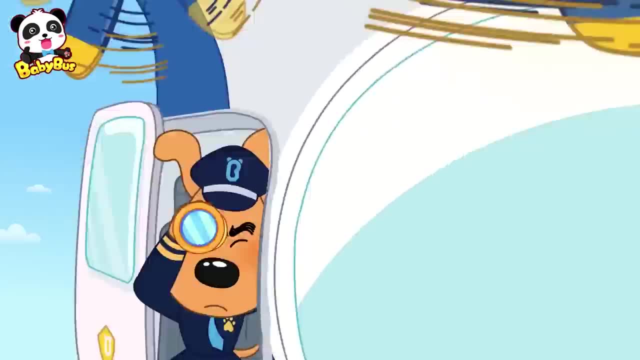 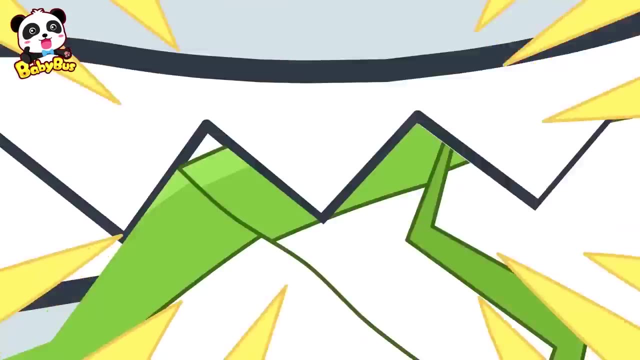 What She had a worst falling out yesterday and my boyfriend is dealing with a breakup. So I'm right here. Don't mess with me, Don't scare me like that vez. Help, He is over there, He's got him. 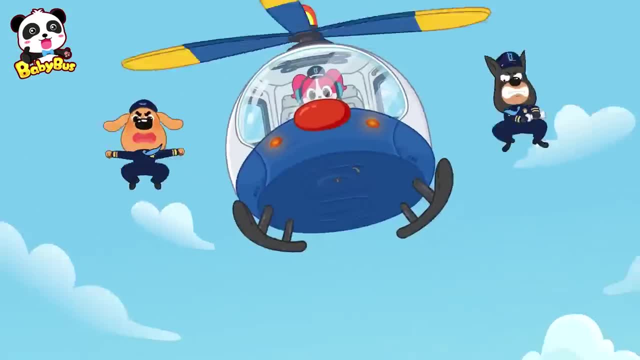 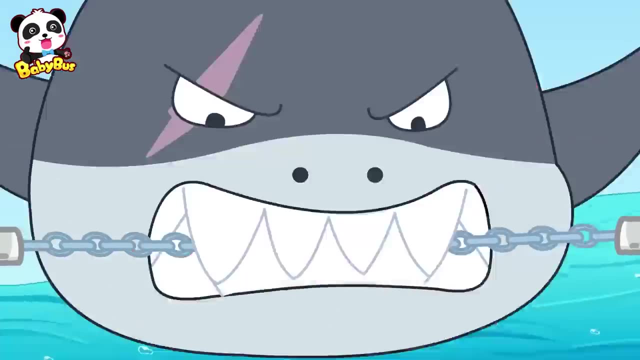 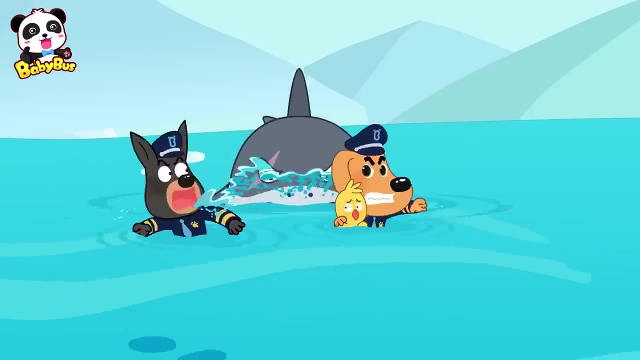 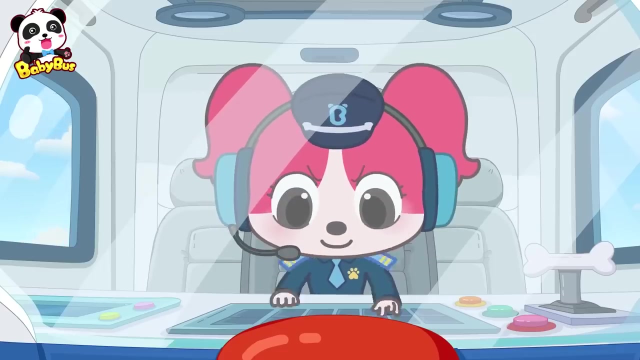 Help me, Help, Hurry. He's in danger. Let's get away. Yeah huh, See what I've got. The shark's so strong. Run everybody, Papillon. we need your help, Got it? Look what I've got. 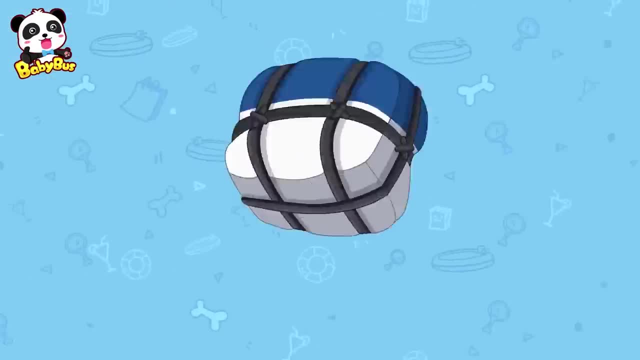 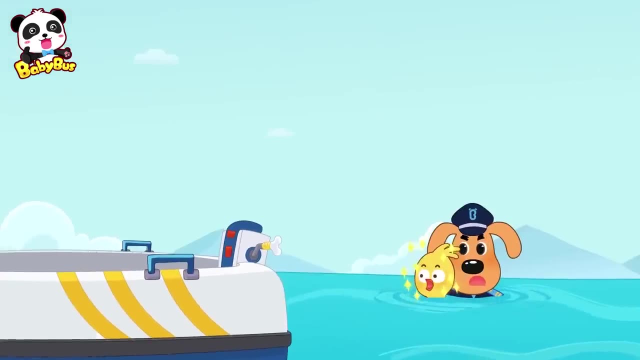 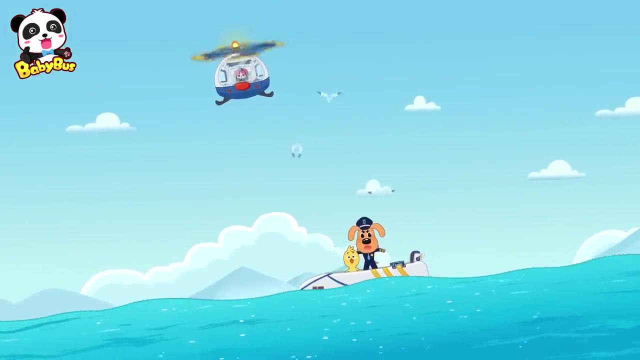 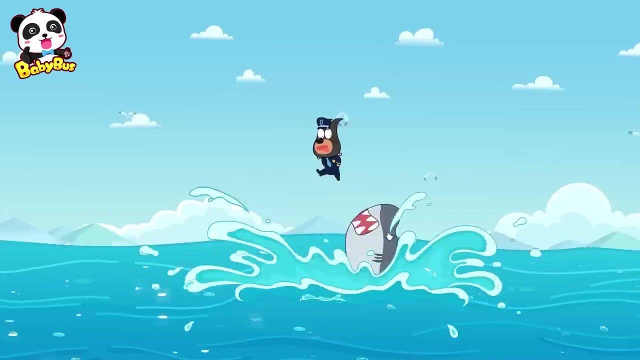 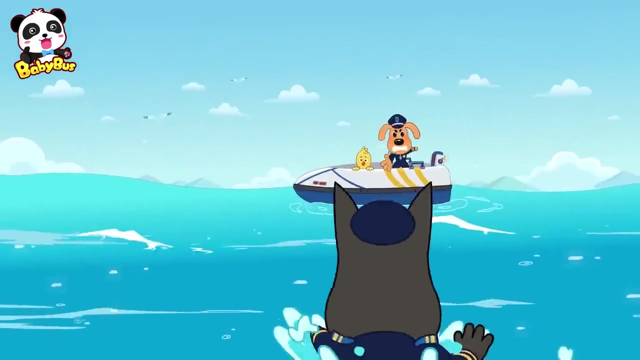 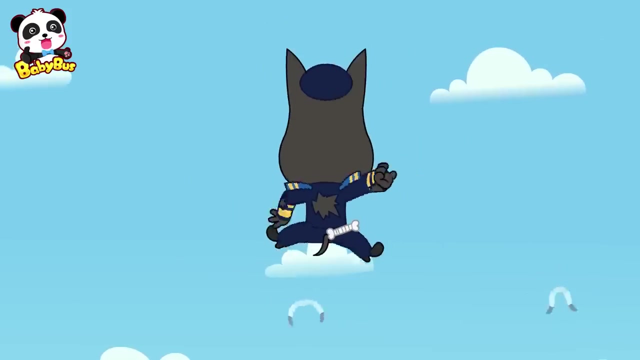 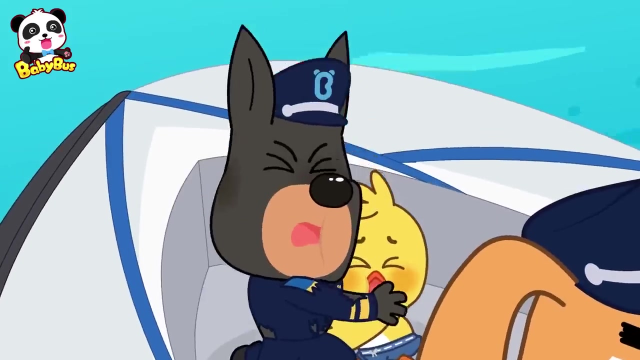 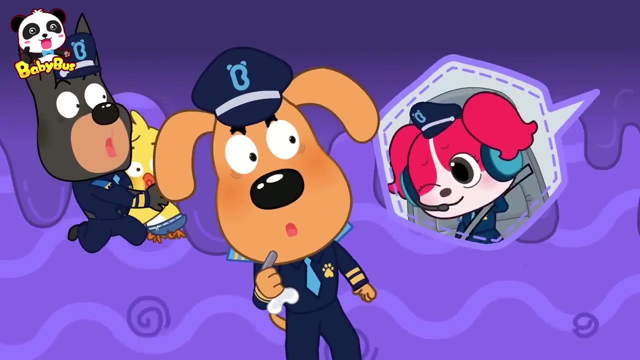 This is the Smart Rescue Boat. It's fully automatic. Huh Whoa, Let's get on. Dobby, hurry up. Oh no, Come on, Hold on tight, everyone, Let's go. I'm sorry, Something's wrong with the welding. 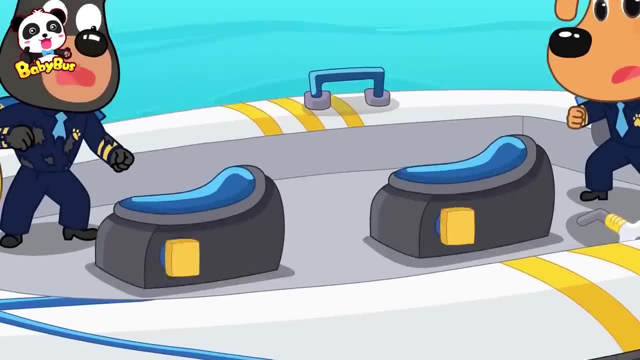 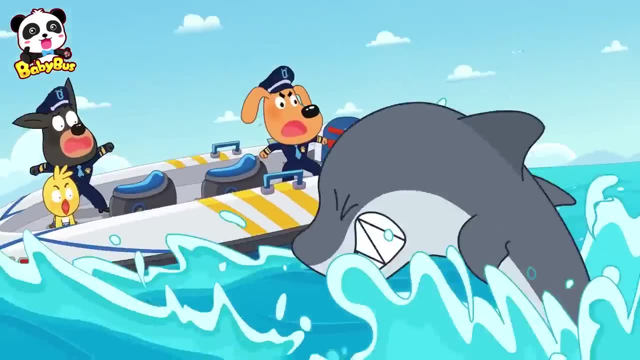 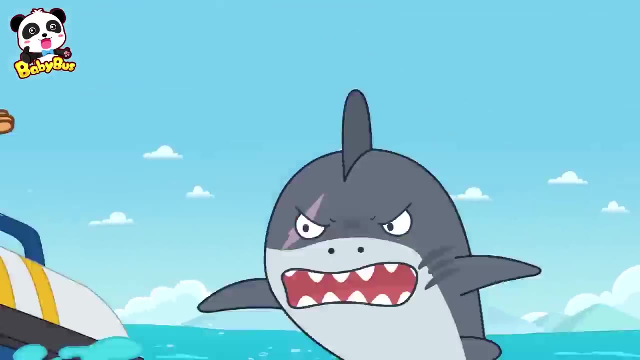 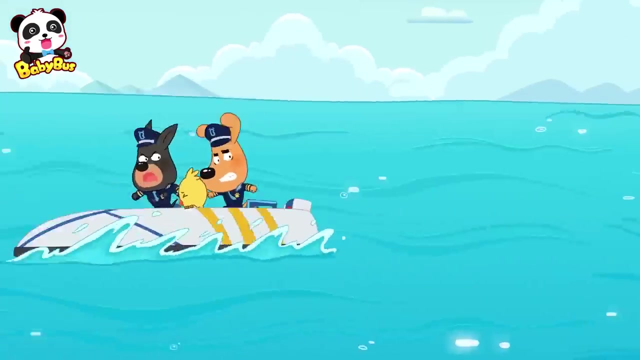 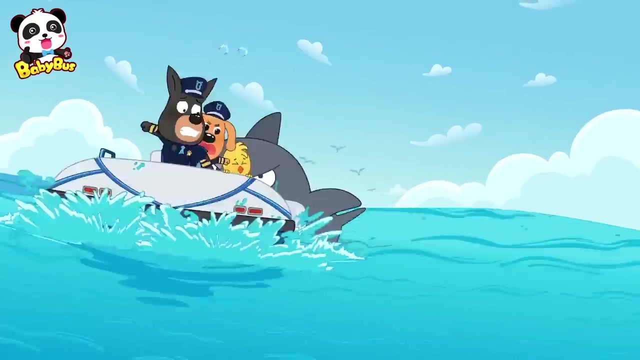 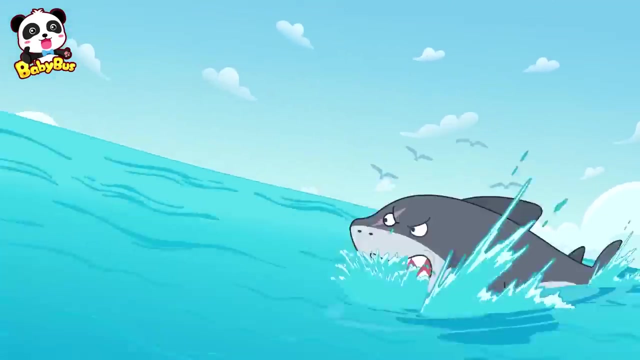 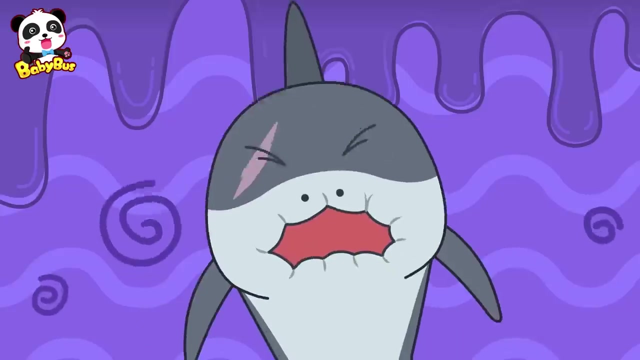 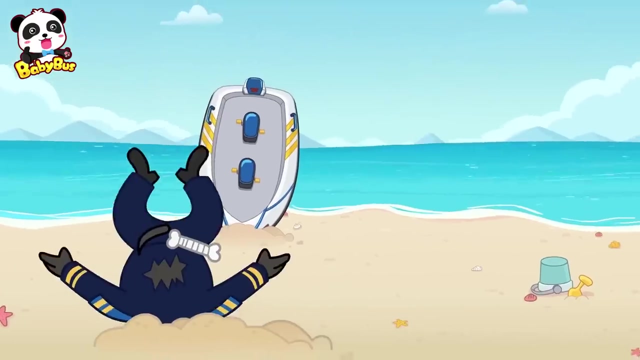 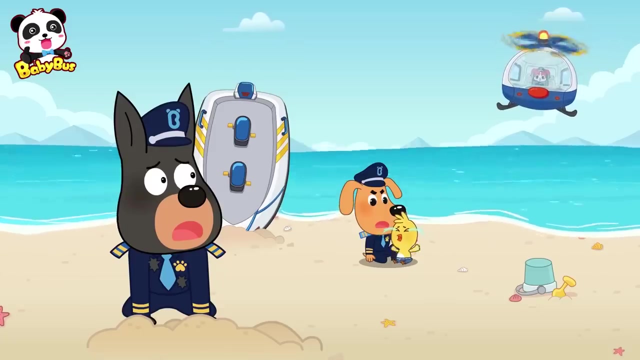 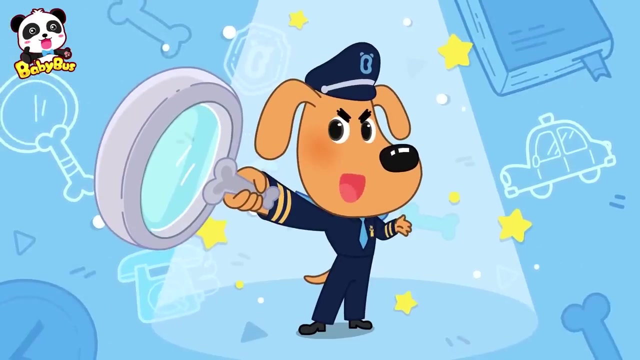 But don't worry, There's another way. Look, Huh, Peddles, Dobby Peddles. Uh Aaah, The shark was so scary. What Sheriff Labrador's Safety Talk. Kids sharks are very dangerous sea animals. 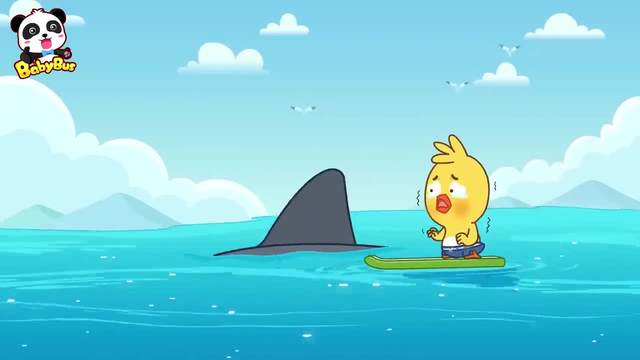 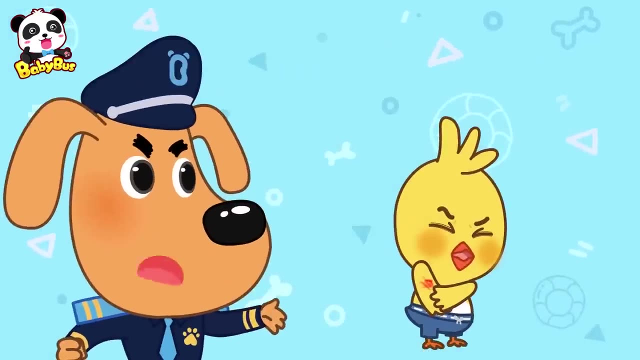 We shouldn't play in the water when there are sharks around. If you ever see a shark, get out of the water and go to a safe place nearby. Also, don't go into the water when you have a wound. The smell of your blood might attract sharks. 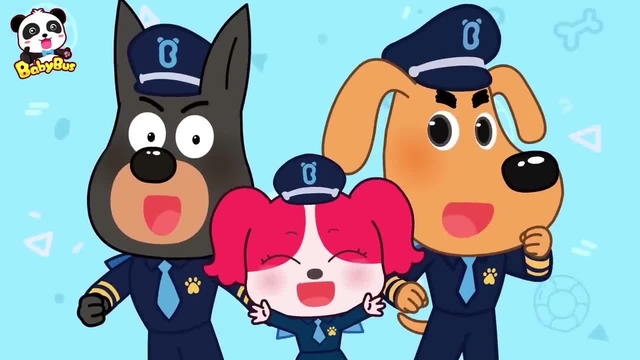 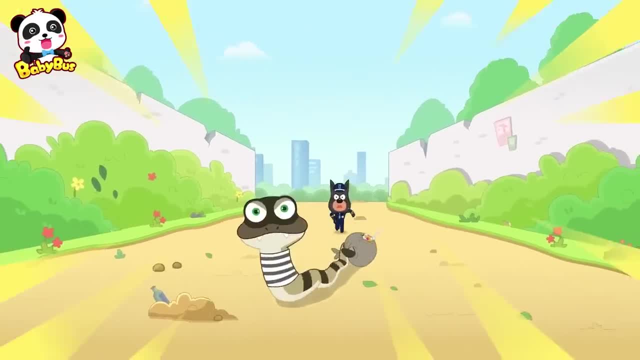 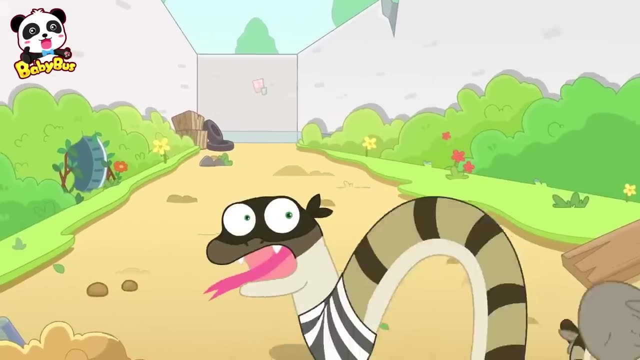 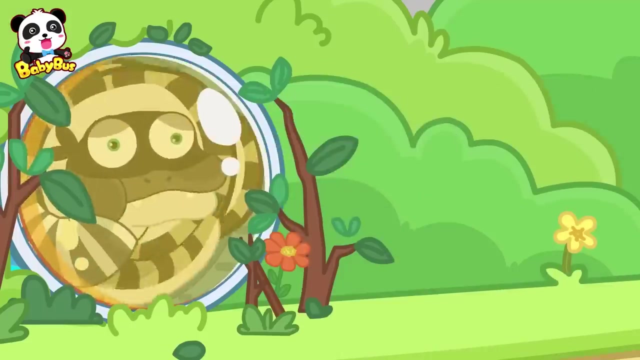 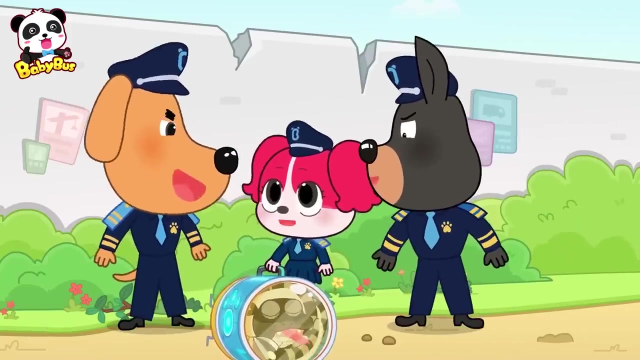 Please remember these tips: Don't play in construction sites. Stop right there, Don't even think about it. You will never catch me. Haha, We got you. Yay, We did it. I'll never steal again. You're going to the police station with me. 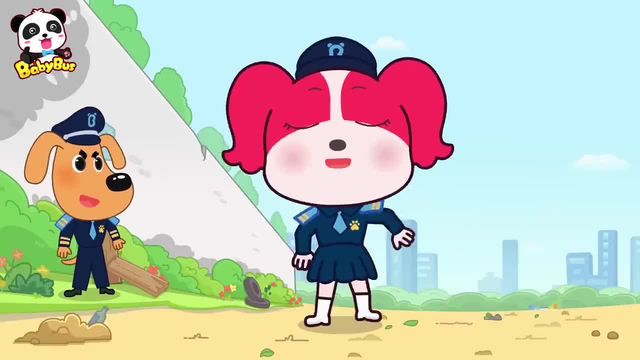 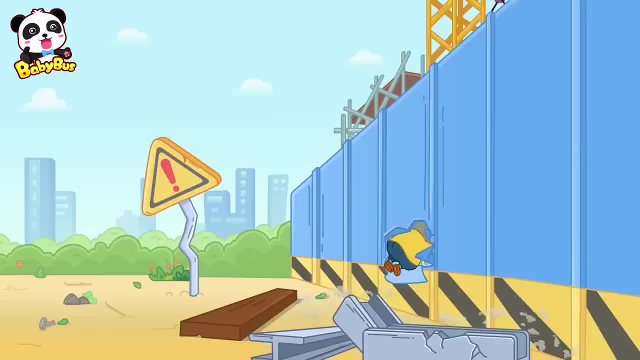 Good job, Papillon. Papillon always has a way. Wow, There are so many construction vehicles in here, Let's go in. Oh no, Little wild geese went into the construction site. It's dangerous in there. We need to get them out. 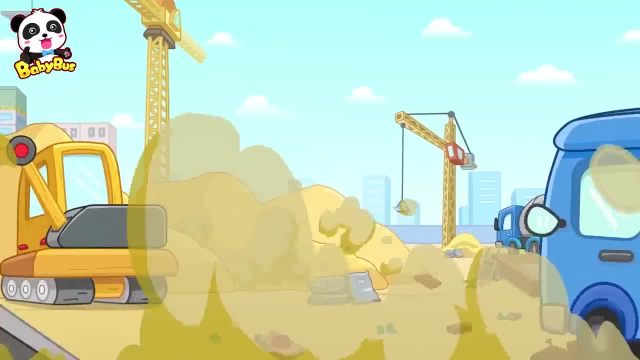 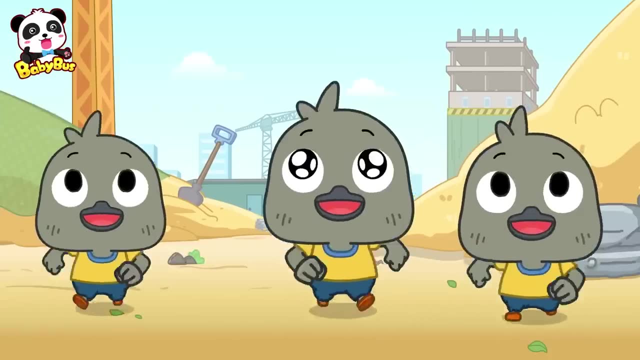 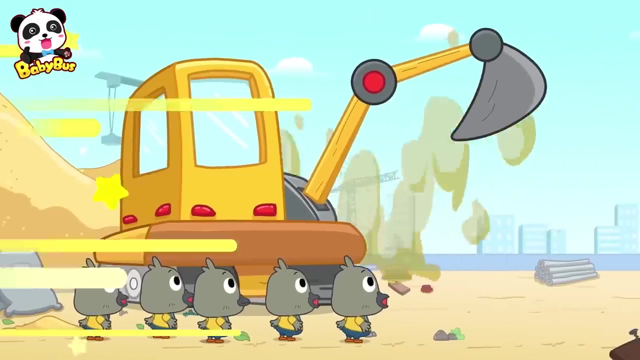 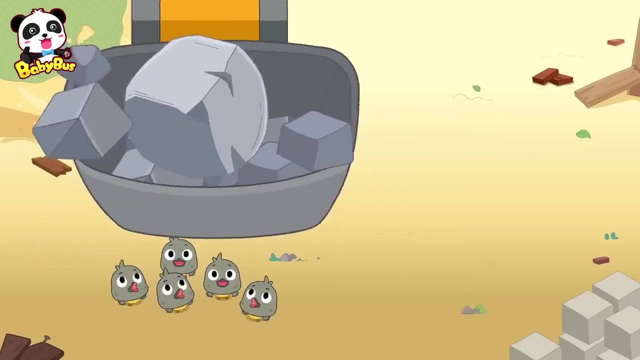 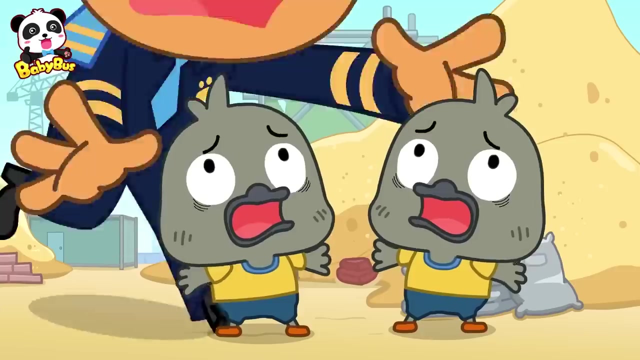 Whoa, Whoa, Whoa, Wow, This is a concrete mixer truck. Whoa, Look, It's an excavator. Wow, It's a loader. It's my favorite. Ah, Watch out, Watch out, Watch out. 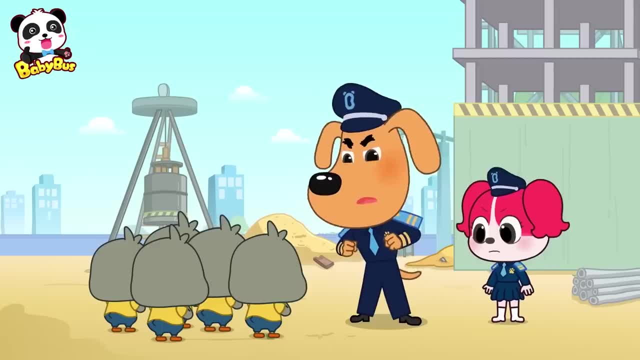 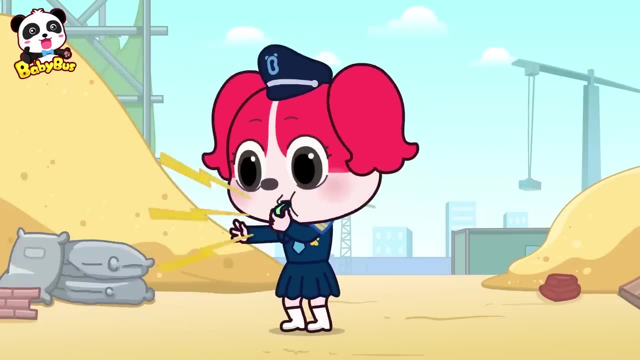 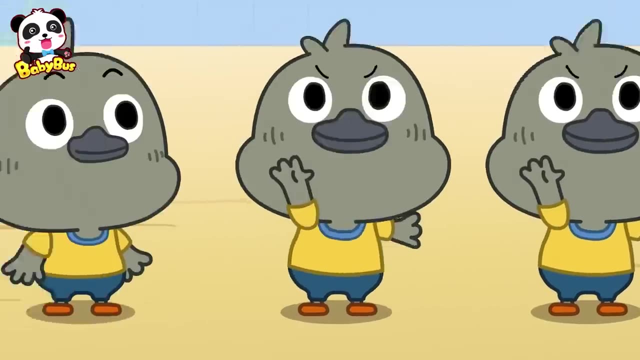 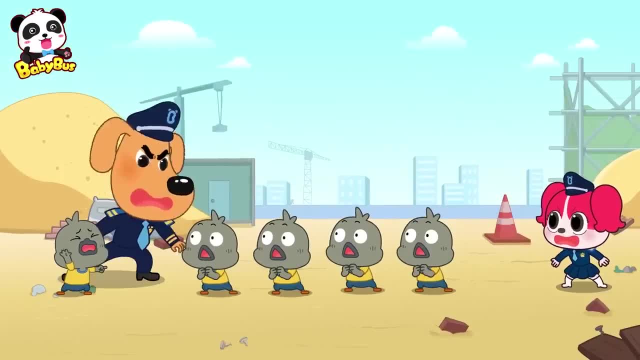 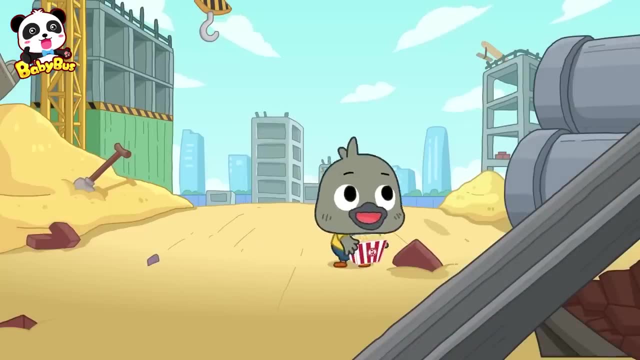 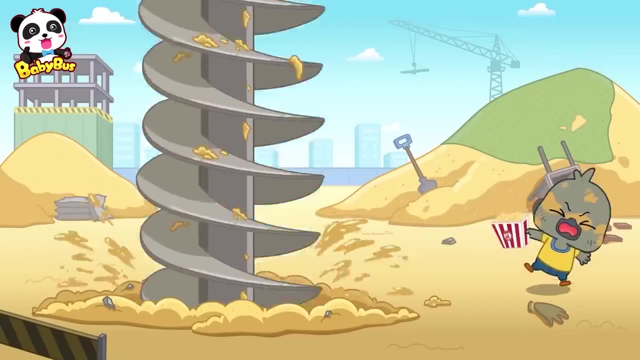 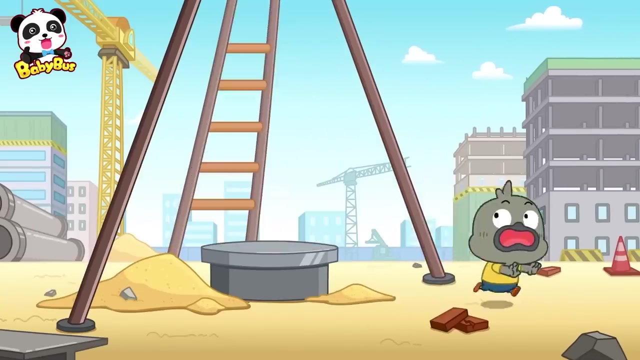 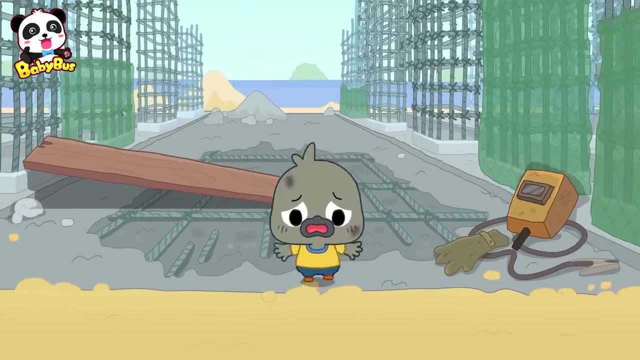 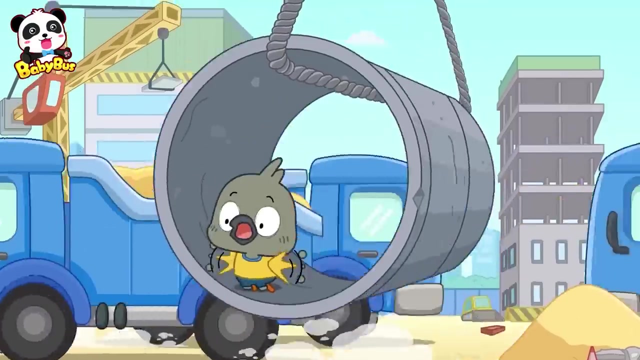 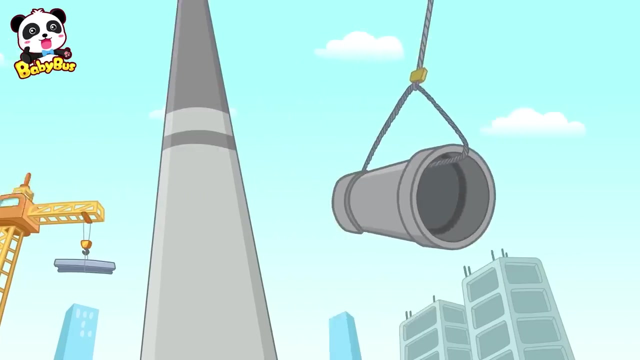 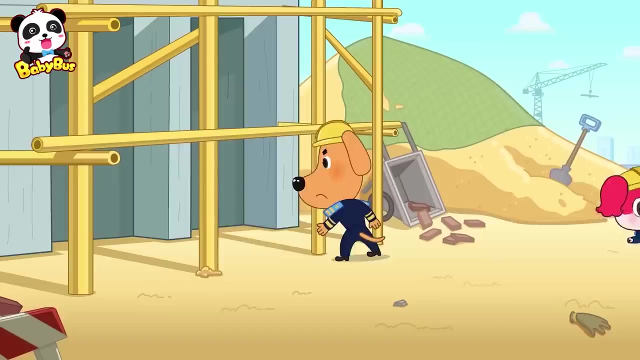 Six Five is missing. We need to find him right now. Wow, Whoa, Wow, It's so dirty. Oh no, It hurts. What. What's going on? Help Little Wild Goose. Whoa, Little Wild Goose, where are you? 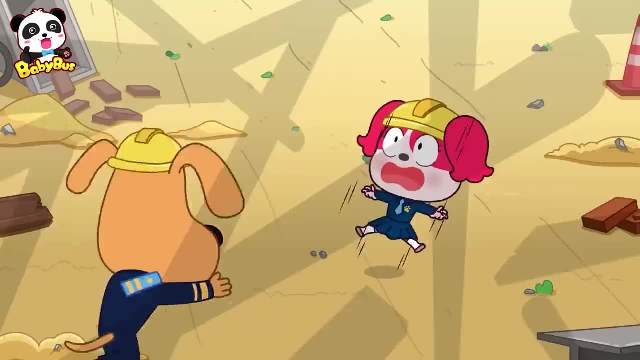 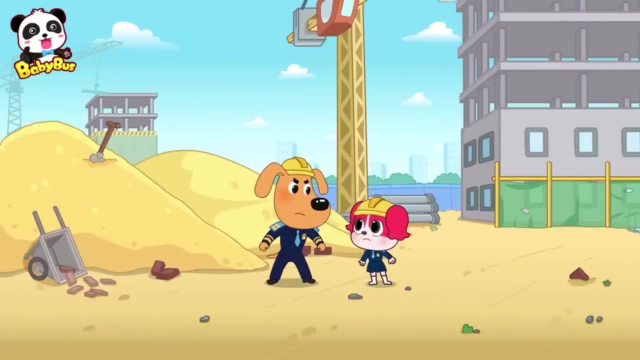 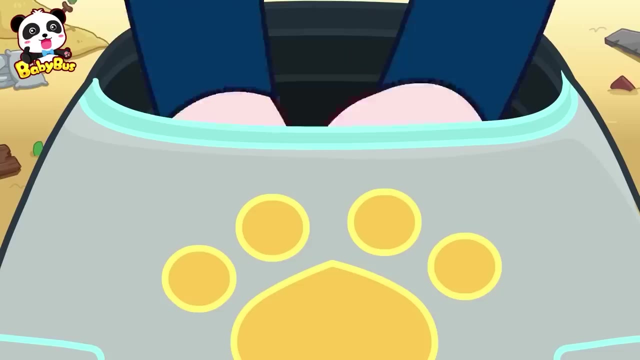 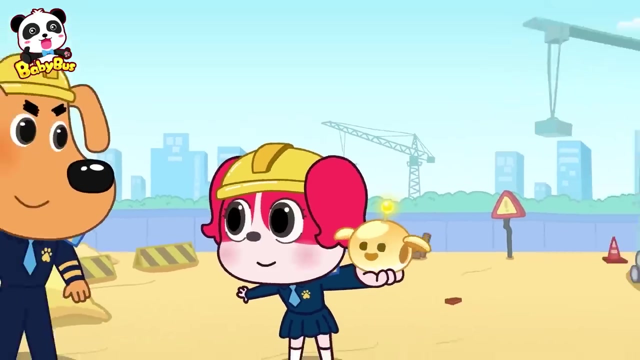 Watch out. It's so dangerous here and it will be hard to find him. We need to use search equipment. Got it, Ta-da, The awesome searching robot, Little Wonton? He'll help us find what we're looking for. 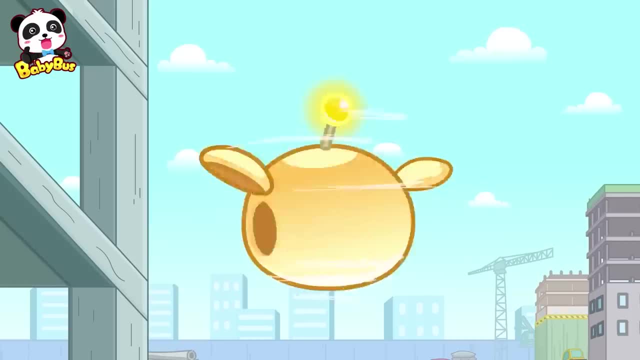 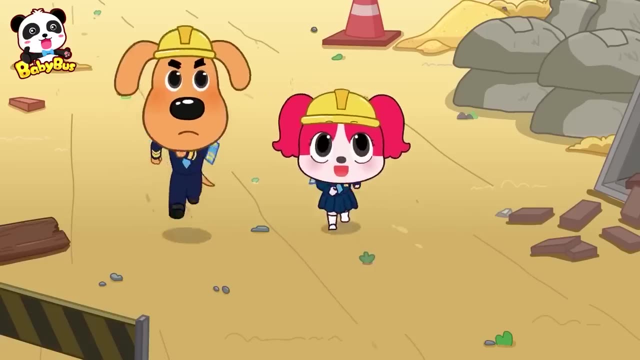 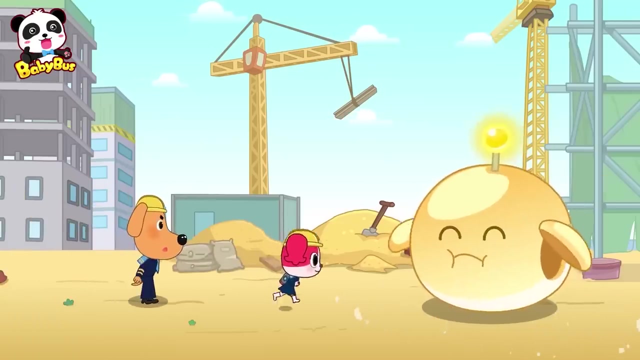 Little Wonton help us find Little Wild Goose Ton-ton, Ton-ton. Little Wild Goose. Little Wild Goose, Ton-ton-ton, Ton-ton-ton, Ton-ton-ton, Ton-ton-ton, Ton-ton-ton. It has got Little Wild Goose with him. 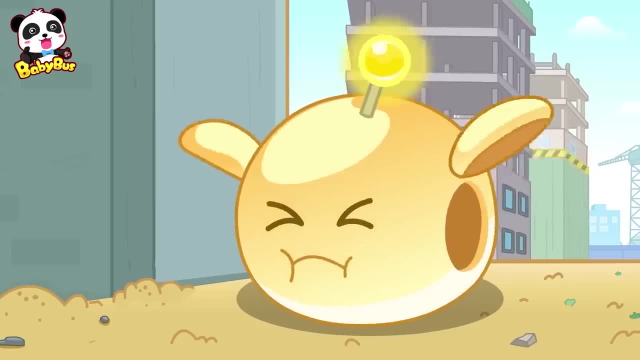 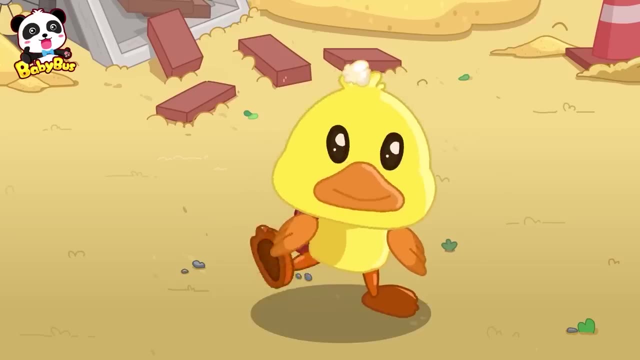 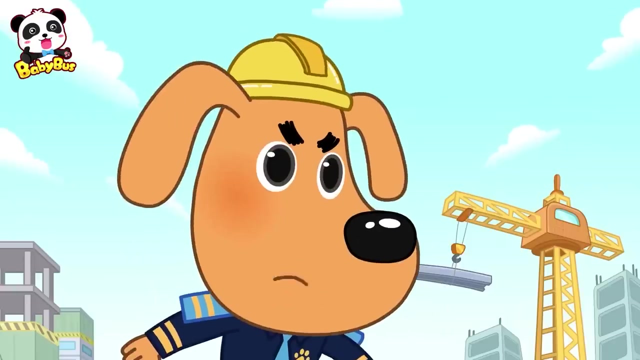 Sorry, he's not perfect just yet. Ton-ton, It must be Little Wild Goose. I am a little dog, Huh. Oh, Hold on Hi-ya-hi-ya-yo Popcorn. Where did you find this? 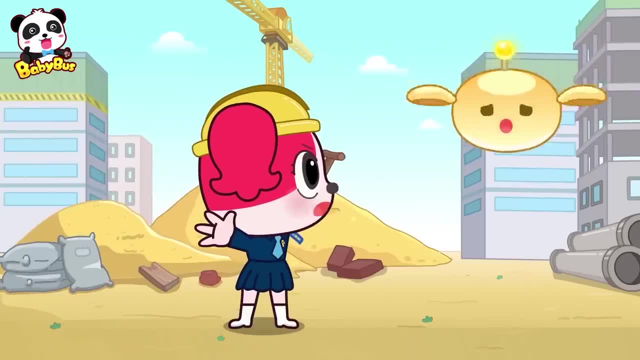 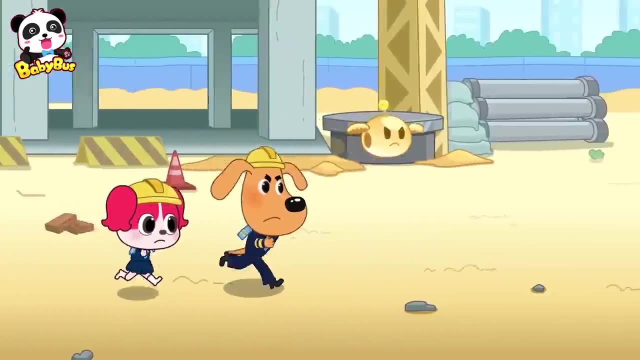 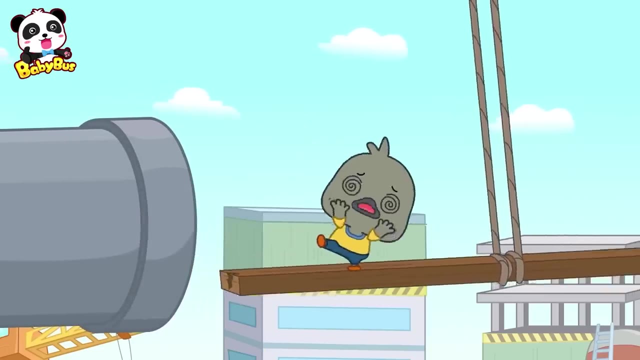 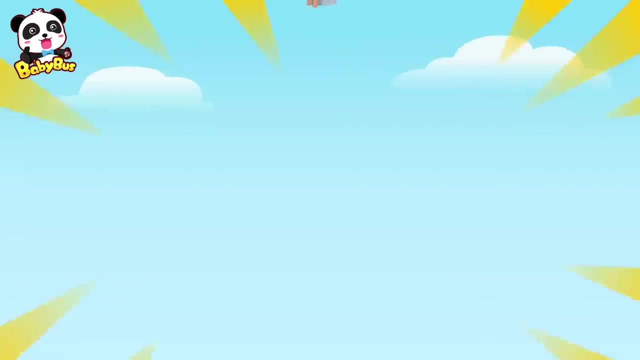 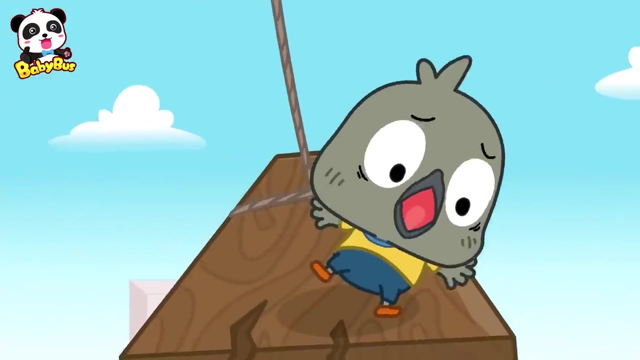 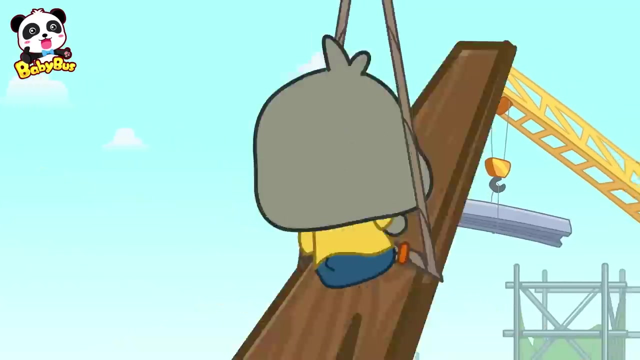 Huh, Little Wonton lead the way now. Oh Ton-ton, Eh Ton-ton, I'm so dizzy, It's so high. Ah, Ah, Ah, Ah, Ah, Ah, Ah, Bwaaah. 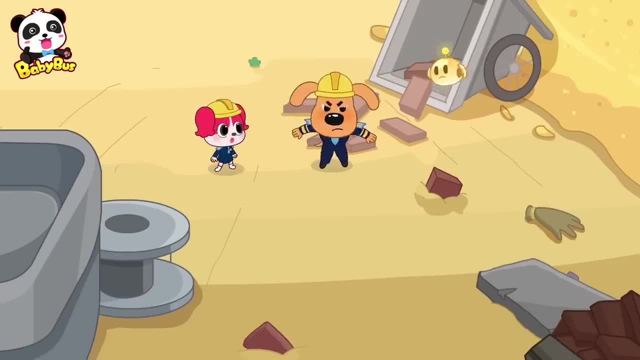 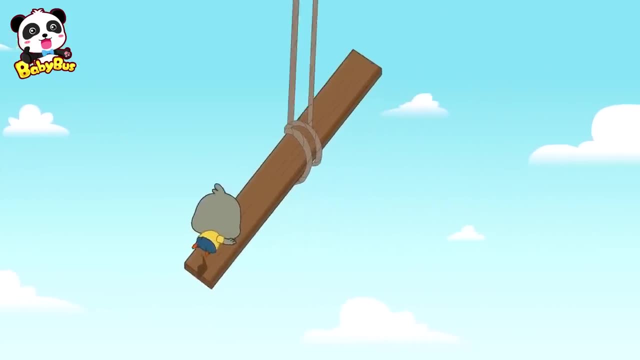 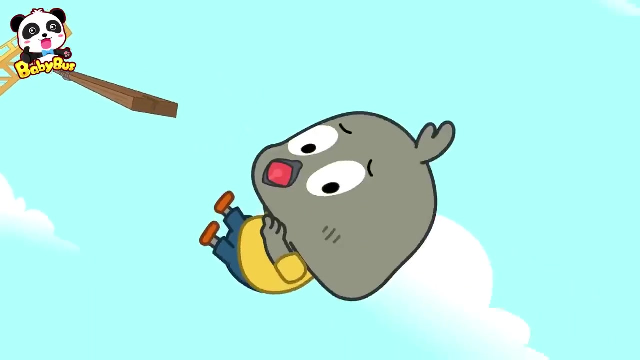 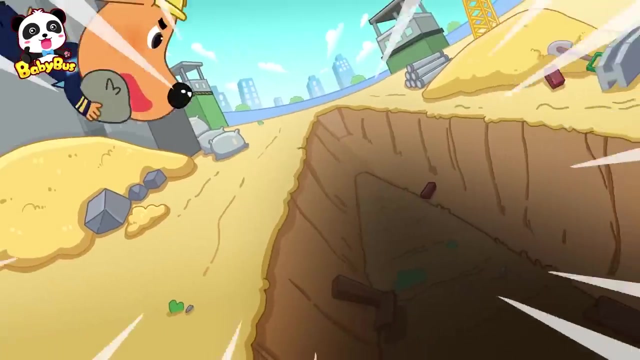 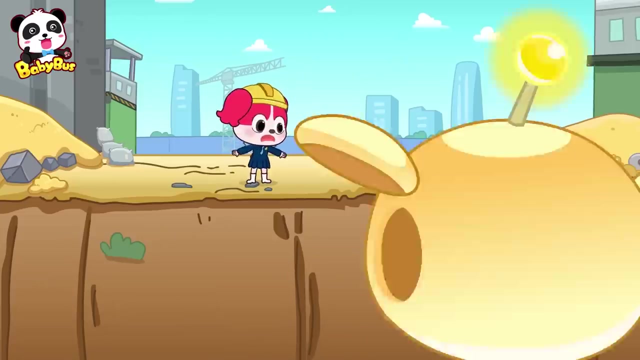 Help me. Huh, Someone's calling for help Over there. Help me, Please. He's in danger. Hurry, Let's go. Okay, Bwaaah, Bwaaah, Sheriff Labrador, Ton-ton Ah. 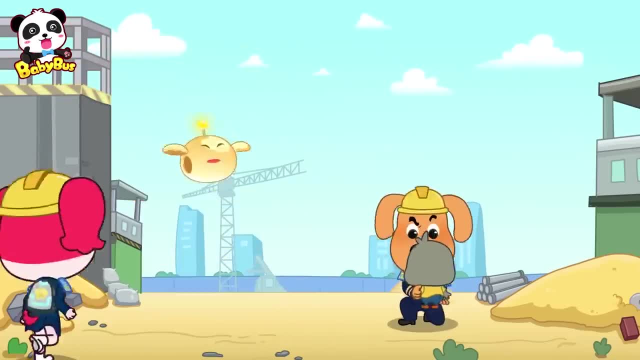 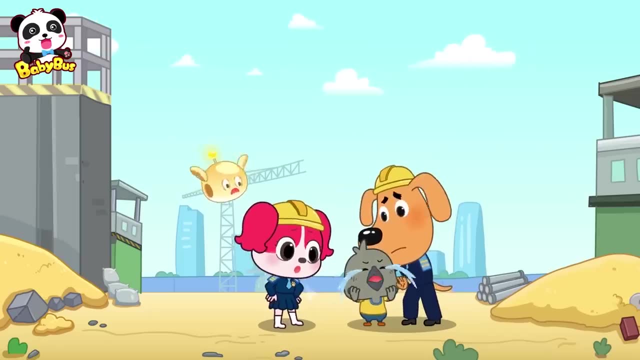 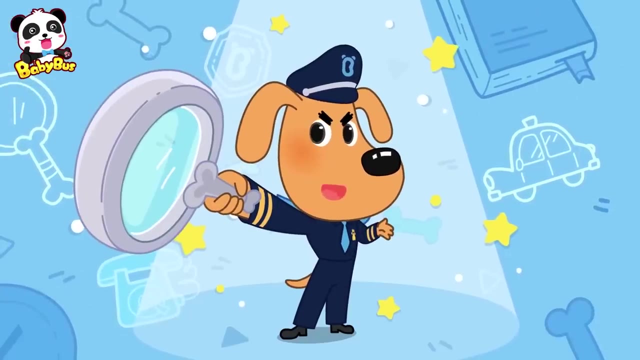 Ah, Ton-ton, We're all right. Thanks, Little Wonton. Ton-ton, That was so scary. I'll never play in construction sites again. Look, Look, Look, Sheriff Labrador's Safety Talk. Construction sites are very dangerous. 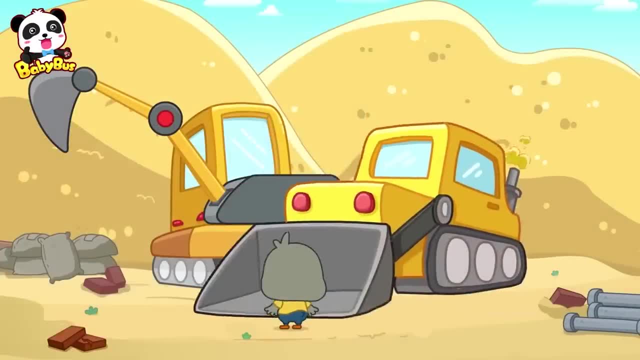 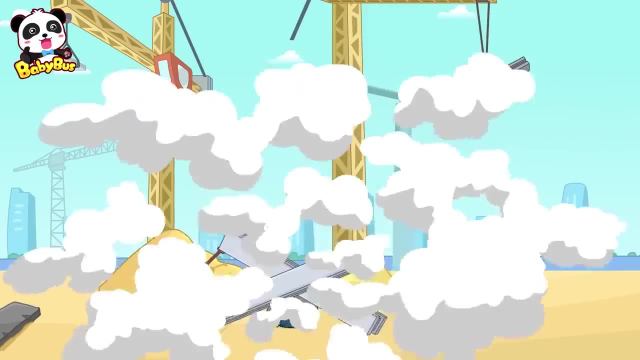 They are full of steels and cement. Construction vehicles often move around. You might get hit and even get hurt. Cranes lift materials up in the air. They might fall and hurt people. There are also big and deep holes. If you get close to one, you might fall in. 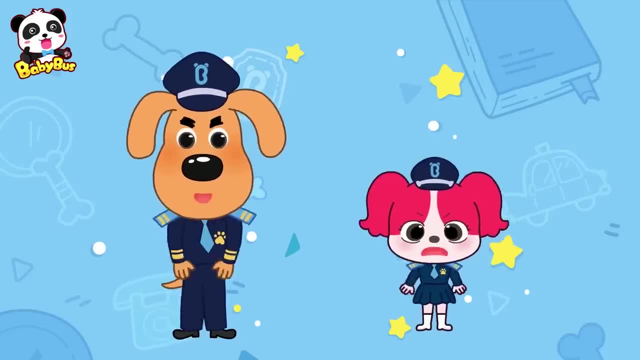 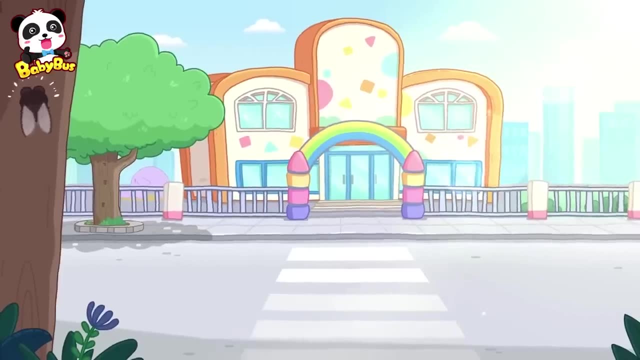 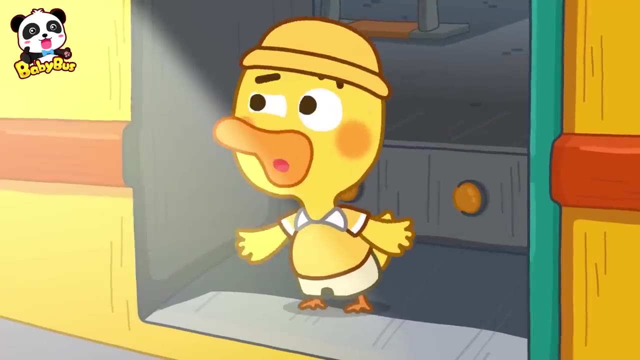 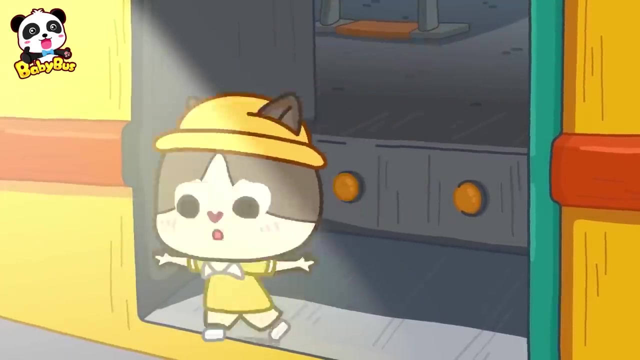 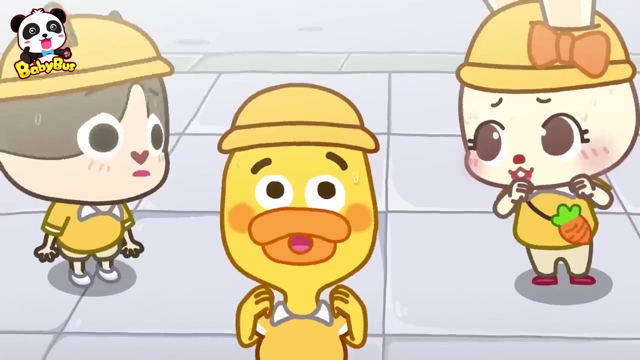 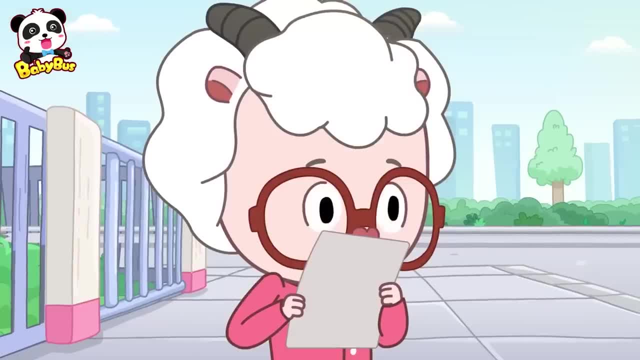 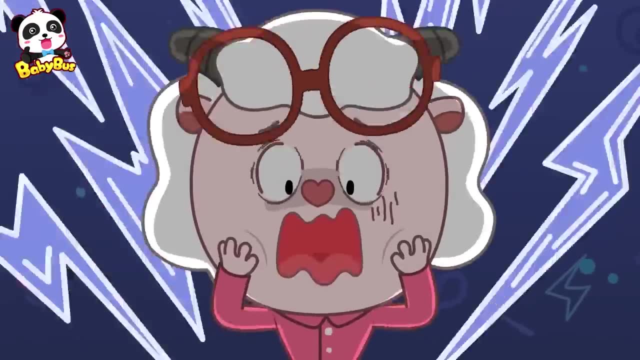 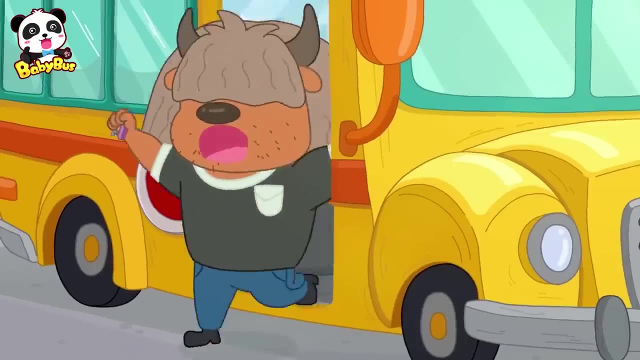 Rabbit Little koala, Oh, Oh, Oh, Little koala. Where is little koala? Hm, Hm, Heu puh, duooo, duuu, puh, duuuu, Oh Oh. 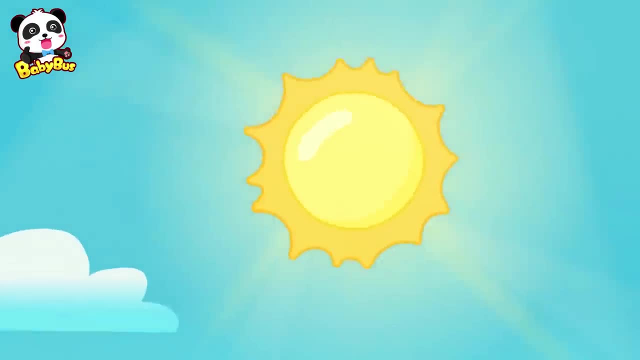 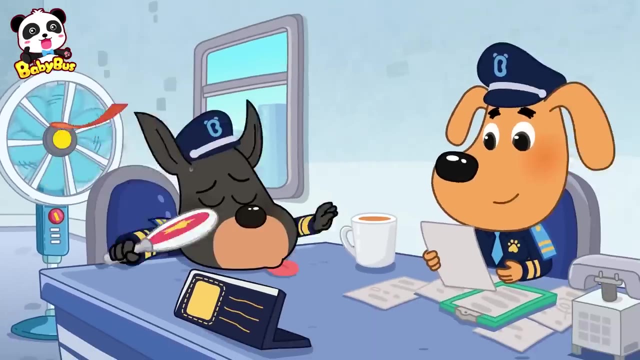 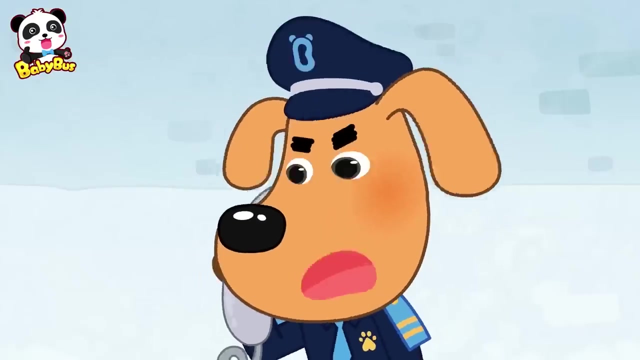 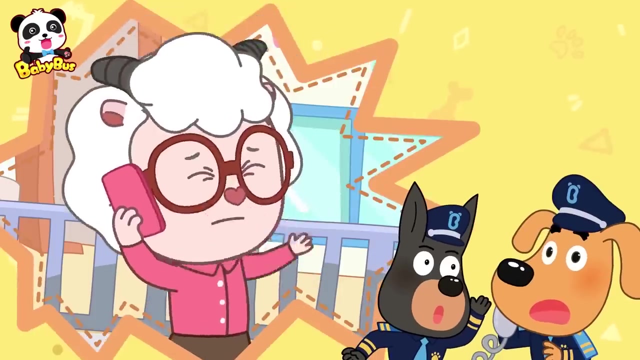 Oh, Oh, Oh. Oh, It's so hot. Dobie, you'll feel cooler if you just relax. Woof, Hi, I'm Sheriff Labrador. Sheriff Labrador, this is Ms Sheep at the preschool. My student, little koala, is missing. Please help. 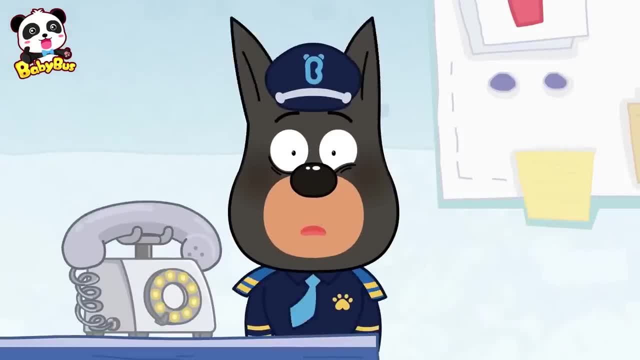 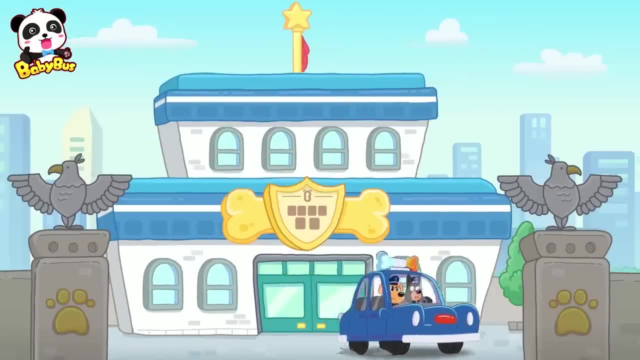 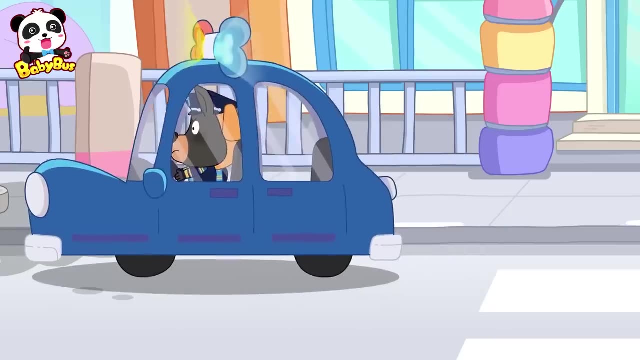 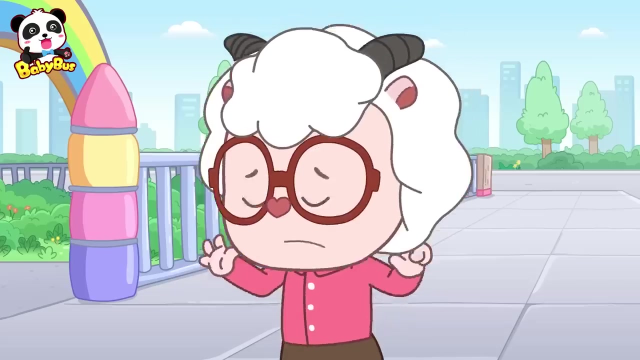 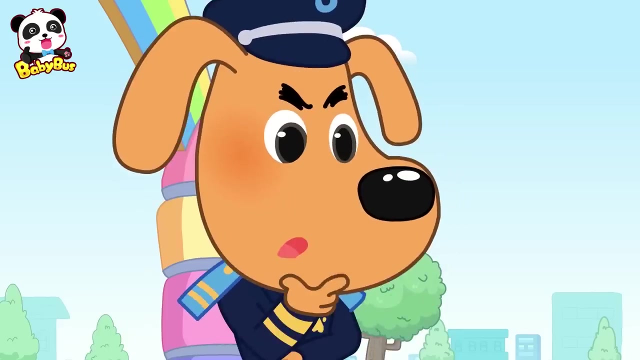 Don't worry, we'll be right there. It's so hot. Ms Sheep, when did you find out that little koala is missing? I found it out when I was counting the children coming off the school bus. What do I do? I see. 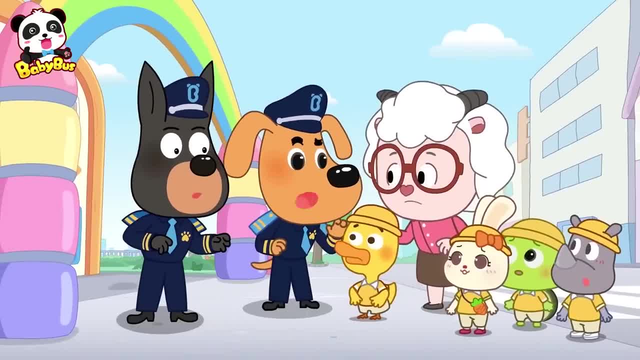 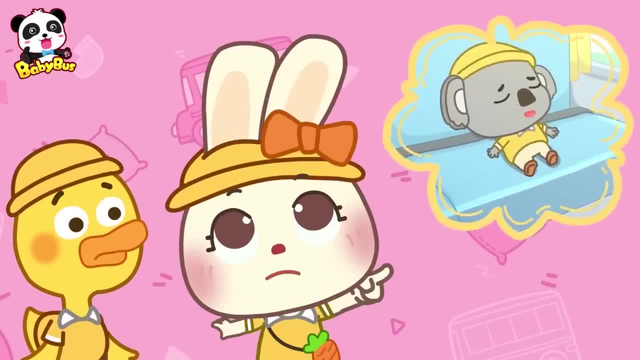 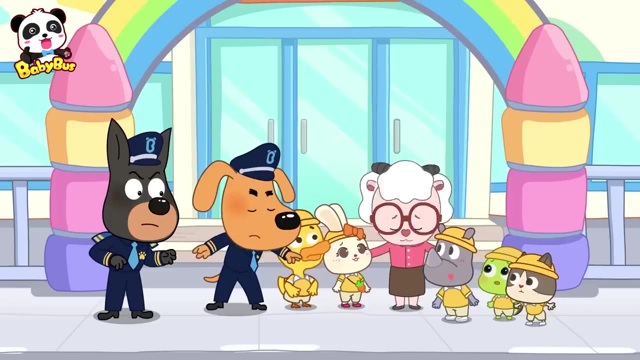 Kids. did you see little koala taking the school bus? Yes, I did. Little koala always sleeps on the bus, Then he might still be on the bus. Where's the bus now? It usually goes to the school bus parking lot after dropping off all the children. 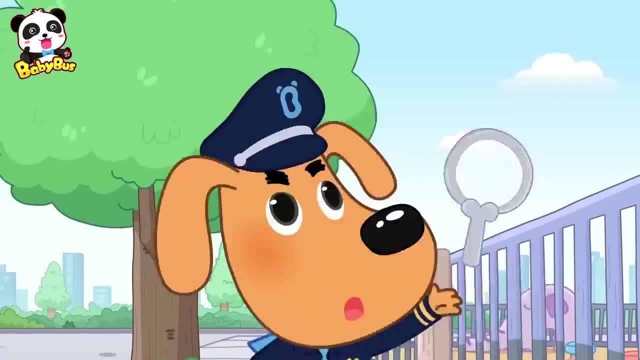 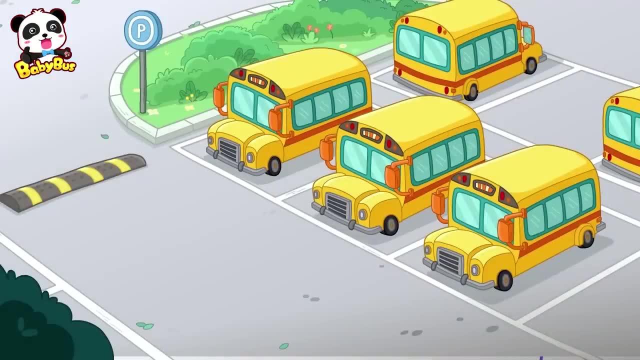 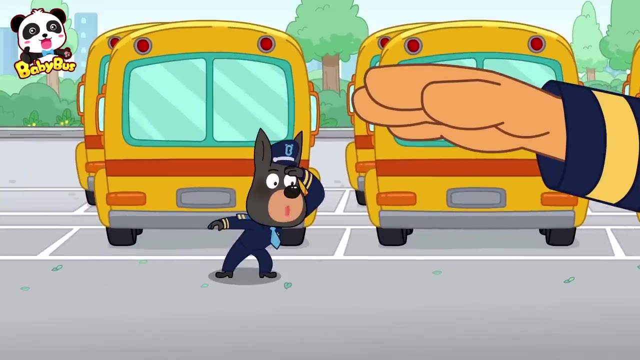 Do you think he's there? We'll go look for him. Don't worry, there's no case that I can't solve. Here's the school bus parking lot. The driver, Mr Yak, might be around here. Found him, Mr Yak? 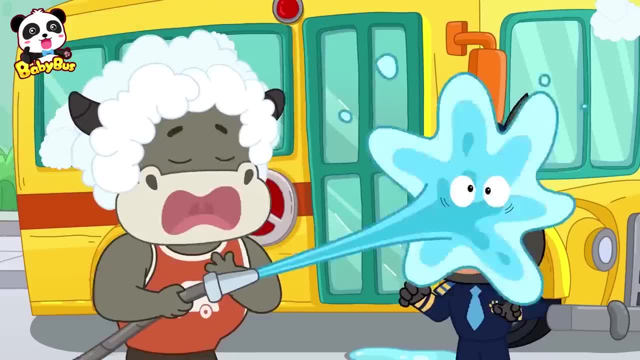 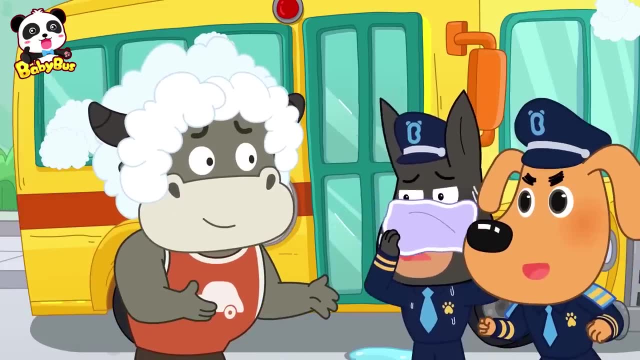 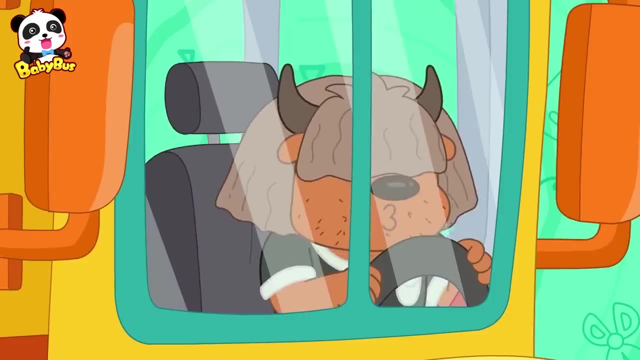 Mr Yak, I'm so sorry, I didn't mean it. I'm so sorry I didn't mean it. You've got the wrong person here. I'm Buffalo. Mr Yak's hair is much longer than mine. Sometimes I wonder if he can actually see when he's driving. 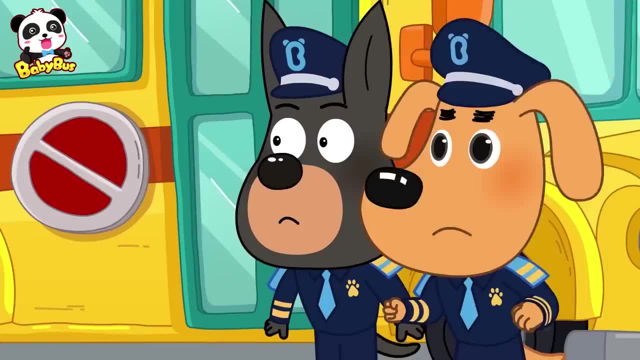 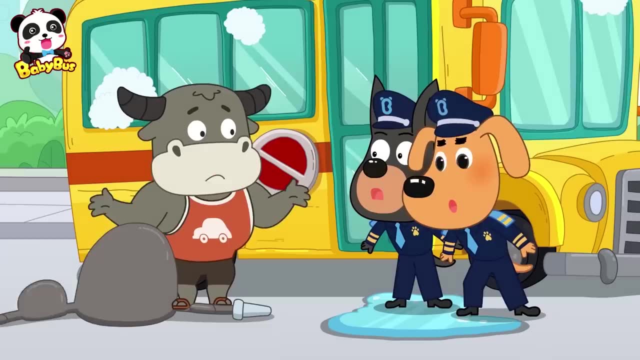 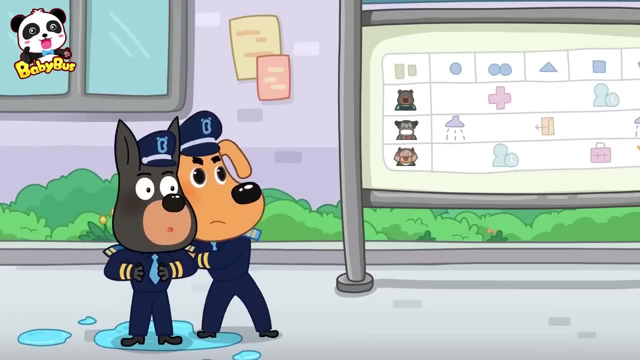 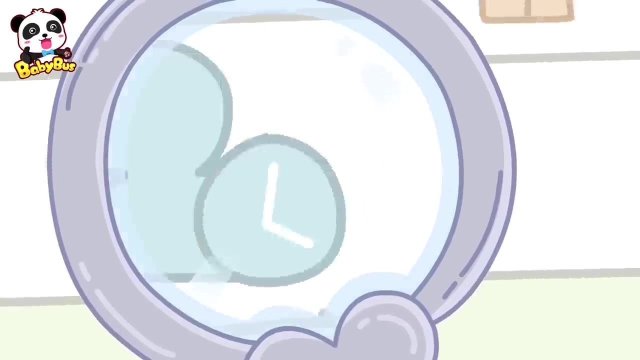 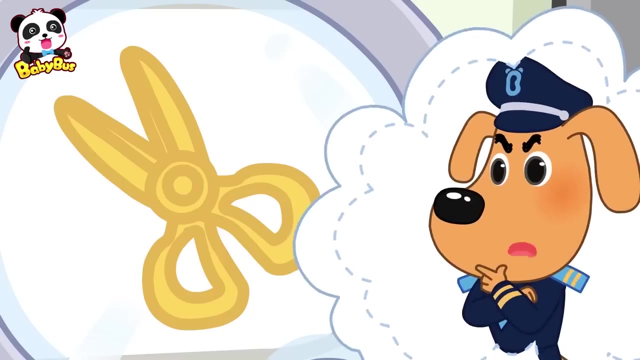 Well, do you know where Mr Yak is right now? No, I don't. His bus is not here. Oh, This is the driver's schedule. This is the logo of the Golden Scissors Hair Salon. Mr Yak is probably getting his hair cut there.